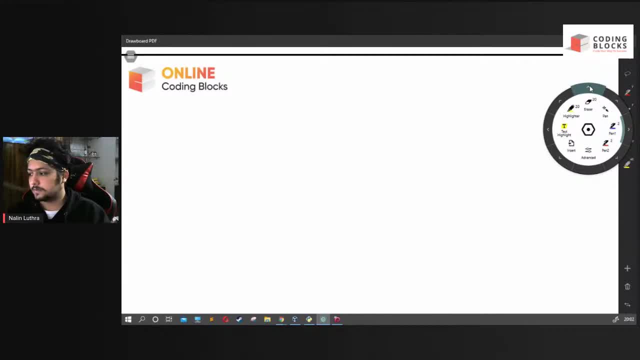 if you don't, I will try to explain it again. Yeah, I went to India watching, That's right, I went to India watching. I told you, like everyone wants to do cybersecurity in the starting that, yeah, we would love to do cybersecurity when actually things get a little bit difficult. 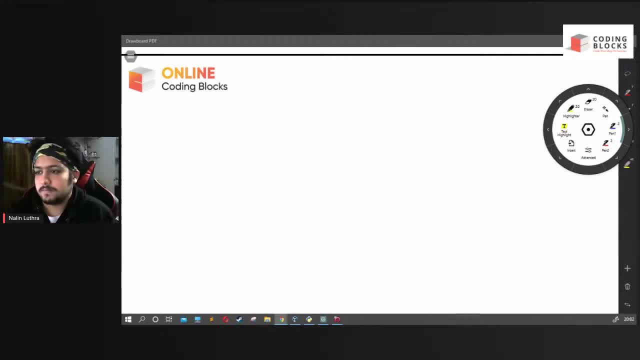 or a little boring, people quit. So I don't know if you guys want to do that. That's your wish, But that's how it goes. Cybersecurity is kind of a mixed field and everything Right. So everyone did understand that. How, why we're using Android. Okay, So let's see. 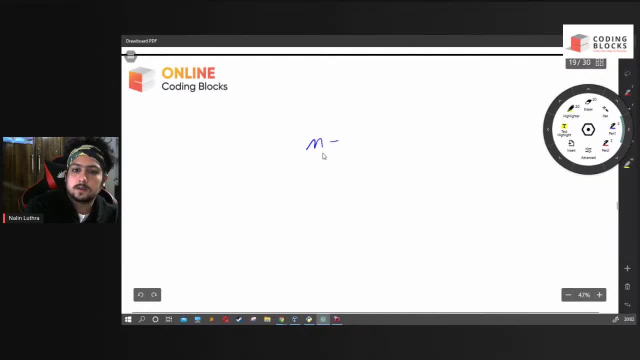 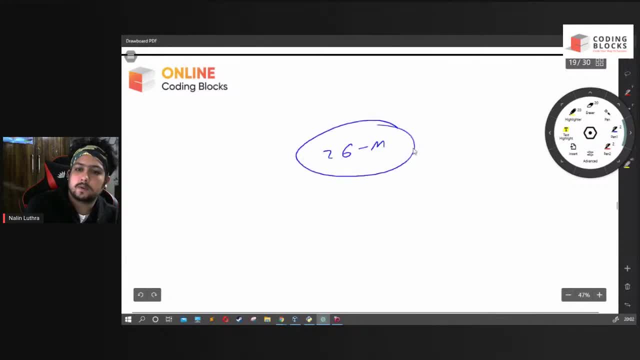 it like 26 minus N. Yeah, 26 minus N. That's why we're using this Right, So everyone didn't understand that Right. Okay, Sounds good, So it looks good to me. Okay Now. 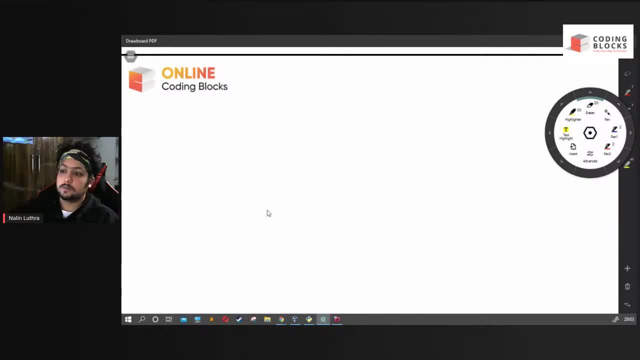 moving forward. I gave a Homebook to one of you guys. Homebook was quite simple. Okay, Let me check that out as well for now. Homebook was quite simple. I gave everyone the homebook guys. so yeah, moving forward on that part. so our homework was that. you need to tell me a method. 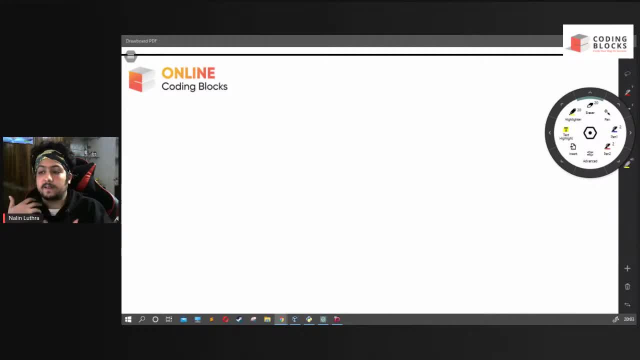 through which you can actually do find a way to decode the ciphers, right? so how would you do that? sorry, one super deal, let's. let's shoot this. so that's how about guys? I don't know, don't say how many have done the homework. that's cool. I don't know who should answer that question. I have good. 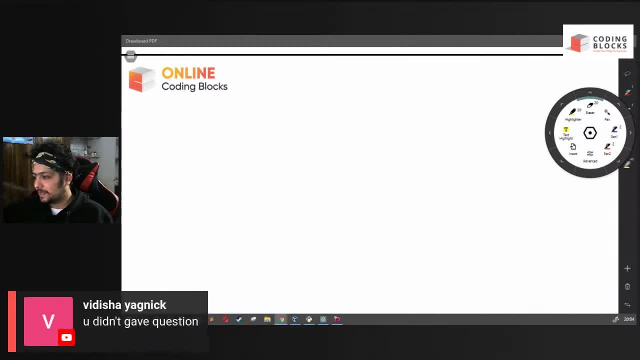 PC, that's good, system, good. I didn't give the question. I gave you, think I don't know how many, if you actually thought about it. so let's come to the point now. so, uh, how to actually decide for the CSI, for that's the point, it's: yeah, are you much you? what did you exactly understand, dude? did you understand the? 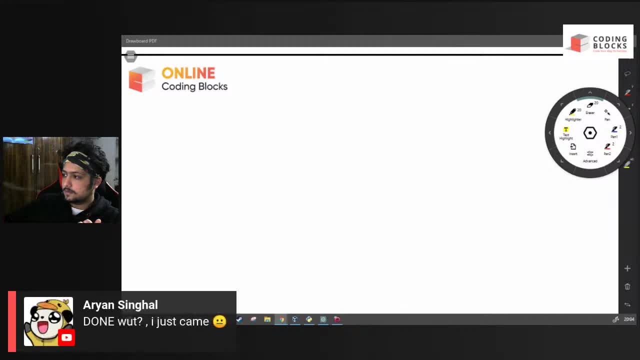 decoding part or what one or any other late, sorry, okay. so a decoder man is think: oh yeah. so, shantha, I will show you how to decode the cipher. okay, so let's come to the point now. so how to? actually I was talking about the point where, uh, how you actually decode the CSI for right, so use the same. 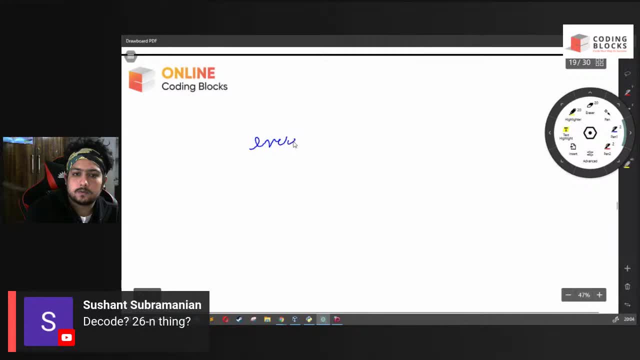 method. as for the encryption: encryption, right, how bad. where you say you want to say a string right along with a key. that's what you give. so, uh, that's what it gives. just to change that part. you change your over here, or n? okay, this is the answer. it gets changed to 26 minus n. 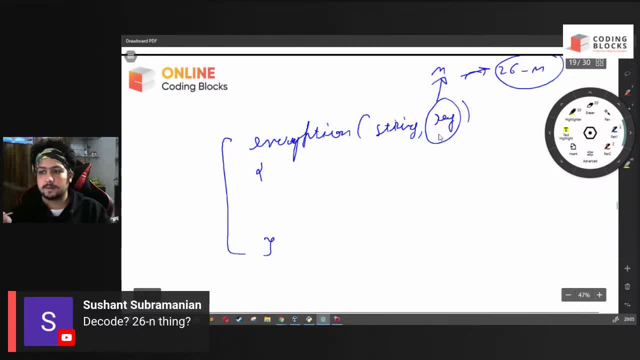 and this will use to be decipher. I explain this thing properly in the last lecture itself. so if you guys have not watched that, you should have. you're late over here. yeah, that's how it is. that's how it is. uh, can you please watch the previous video, because I explained properly over there. 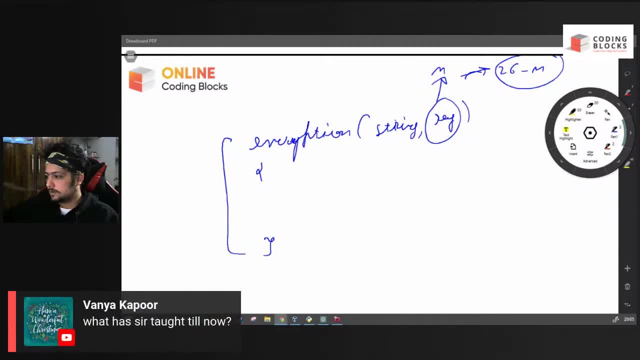 because everyone didn't understood that uh I have when I have not taught anything. I'm just explaining what I said in the last video because many people are saying I didn't understand why we use 26 minus n. so we're using 26 minus n is because uh, 26 is number of alphabets we have. 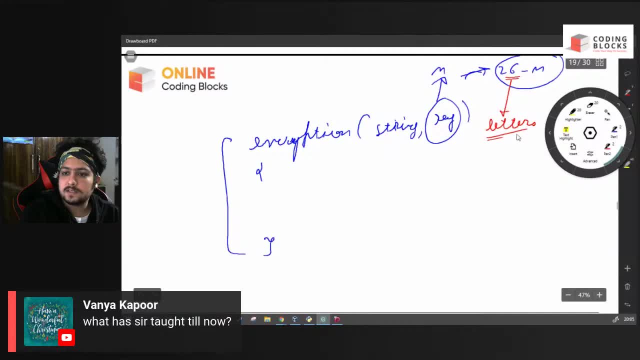 like: so, let's say letters. so it's kind of a simple thing that when you have these letters and you say, uh, let's go. okay, let's say we have abcd and that's just four letters we have. let's imagine for a while that whole English is only based on four letters: a, b, c, b, that's all okay. uh, let's, let's get bottom. 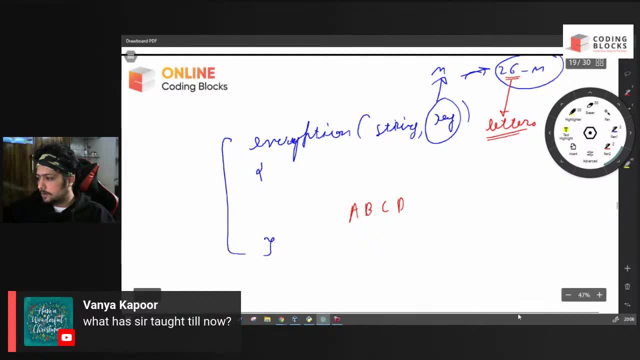 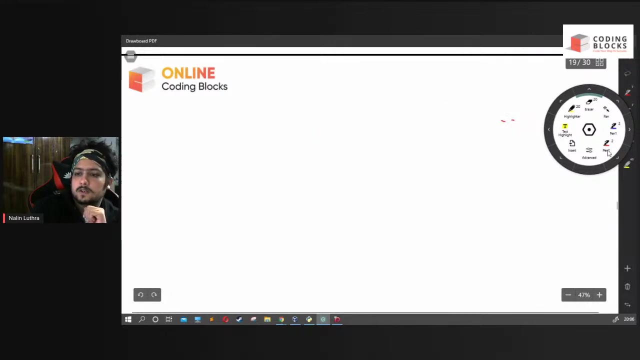 of the point and let's understand once and for all. okay, uh, okay, code again. okay, I will do that. I will do that. give me a five minutes, okay. so let's understand that. let's imagine that whole English, what we have learned or whatever you know, is not there. okay, let's say, the whole English is only based on four letters. okay, 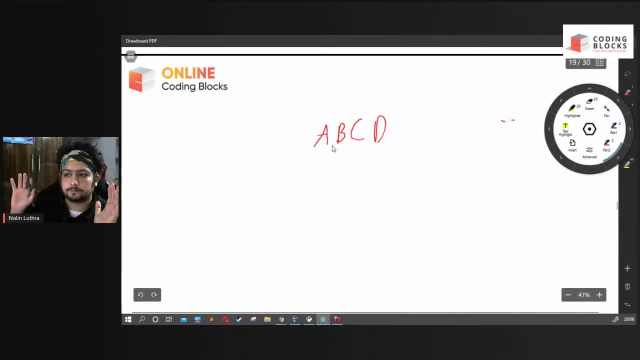 a, b, c, D. that's all. whole English is based on four letters- CD. now when I use a c cipher on this and say the value of n is 3, so what happens is I get something like this: a because it's 3. so I will start from D, a, B, C, D. 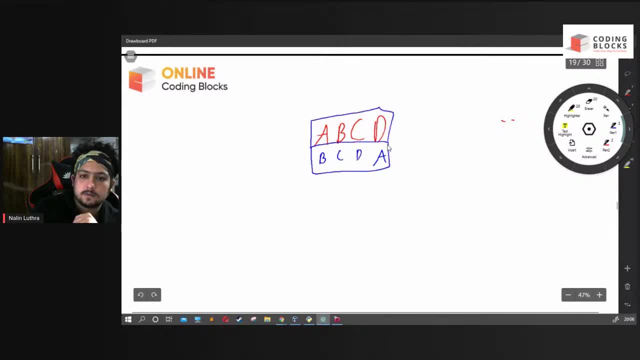 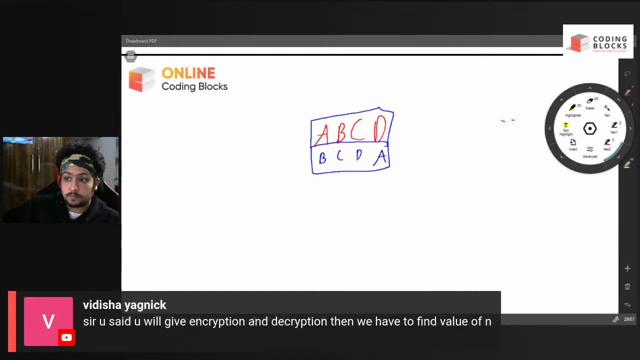 right, this is what I get from this. if it's only based on four letters now, just imagine, on this part art, I completely switch it, okay, yeah, I did say that I'm gonna start that just right now, which will have not done anything much. I'm just explaining what I explained yesterday. the small example, that's all. 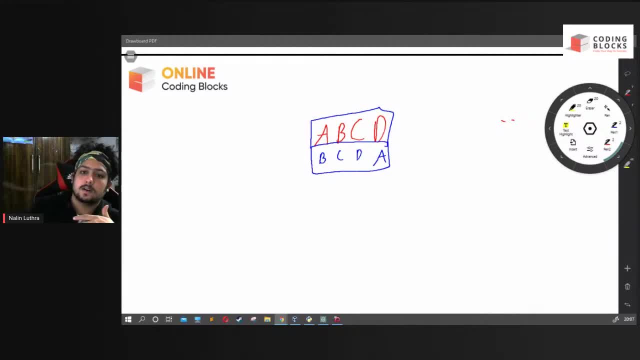 don't worry guys. okay, so come to this point is now that we have a, B, C, D. so if- let imagine, if we just got four letters in English- yeah, maybe CD- what we'll have, say n is equal to you 3, we will have BCD. right now, when we want to decrypt it, what you will do is: 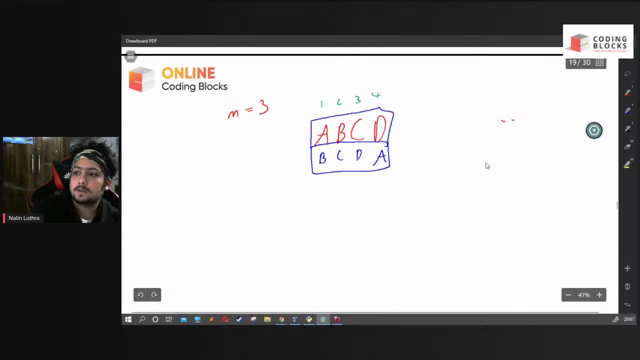 you will just say: okay, we got 1, 2, 3, 4, simple, just say 4 minus n, and over here is 3, so we say it's equal to 1. so now n is equal to 1 and rewrite it. so what happens? if n is equal to 1, what we get, we get a, B. sorry, what we get, n is equal to 1, we. 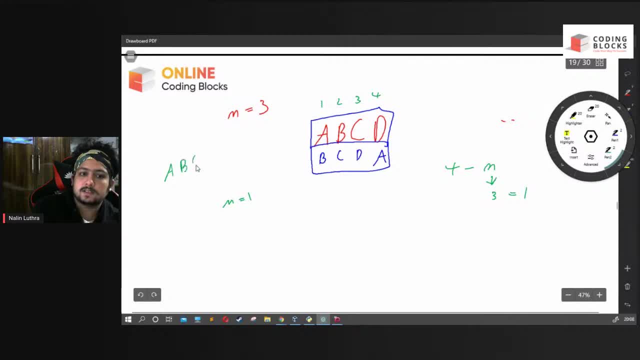 get over here. so, for example, we want to code ABCD itself. what do we get from this one? we get BCD right. this is what we get. now I want a gain ABCD back, like this is what I want. so how do I pair it? I want B to be a right, so what I do can simple: n. 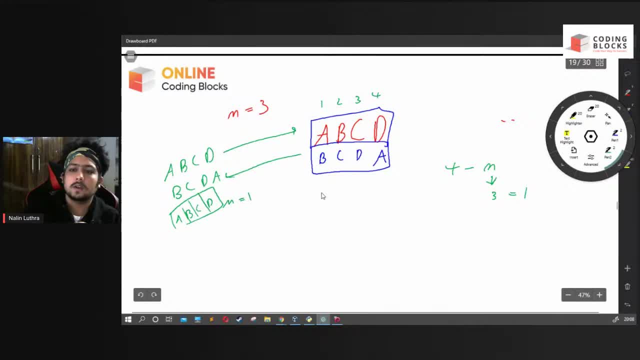 is equal to 1, right, so what I do- mosquitoes- okay. so in this case, n is equal to 1. you, yeah, that's a smart option, thank you. thank you so much. okay, so we have ABCD: n is equal to 1 and what I do? I just want B to be a right. that's how it is so. 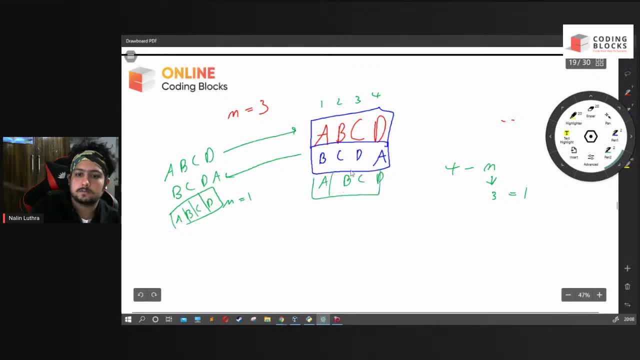 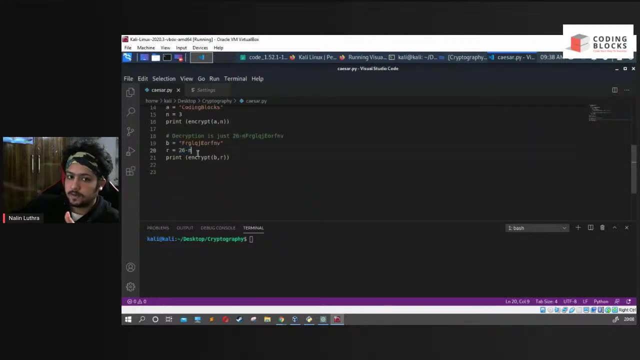 A, B, C, D and it works. that's all right. so that's just reverse. n is equal to 1. think cool, okay, this is what I've done right over here, if you guys can see it right. I said 26 minus n, right, and I did everything the same. it's working fine. 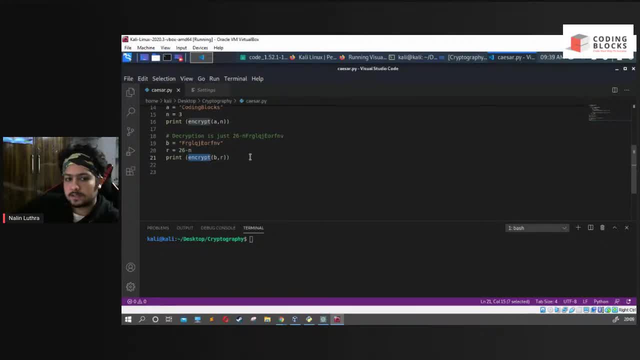 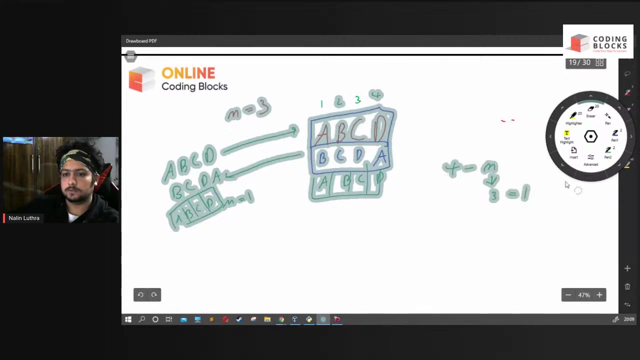 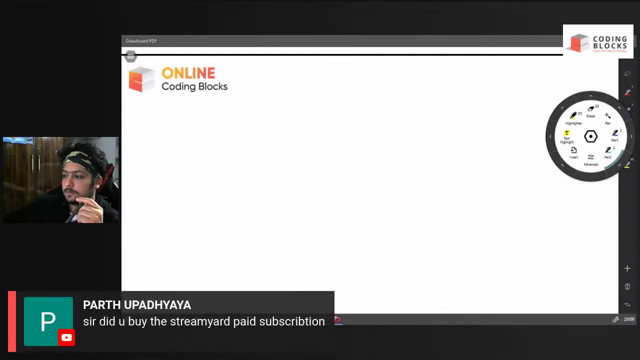 that was supposed to work right, like that's what I'm doing. that's how the question works and that's how encryption check cool, so let's put all together. if cool, cool, great, yeah, we guess. so, yeah, we did. okay, please zoom. okay, I'll zoom when I start to. 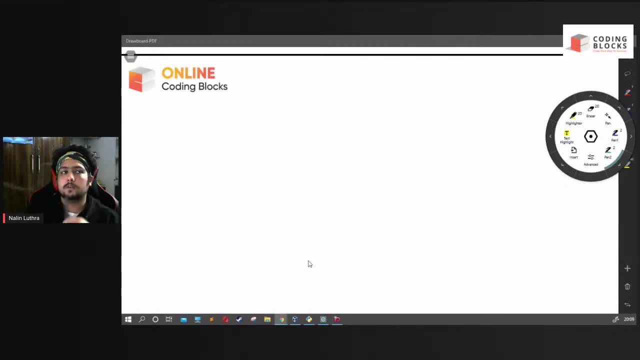 program. now the question is, what if you don't have the key? and what is the key over here? key is the value of n, which we require to actually decode the message. what if we don't have that key to actually decode it? now, now that something comes over here interesting, the interesting part of the whole, 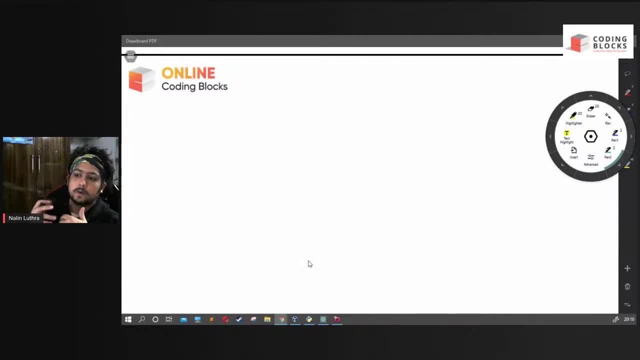 scenario is that when you want to actually decode the message, what you do you simply find all possible strings which are which can be made through that. and what are those possible strings? there are only 26 possible strings because that's can be the value of n. right value of n can only be as big as 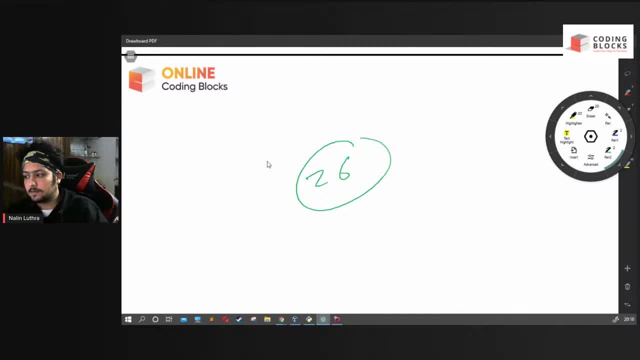 26, right, and we're good to go. so what I do is I will make a small loop for, for int, i is equal to 0. we say i is less than what? 26- okay, let's say it's 1, that's right. we say i plus, plus, that's all, and we use the. 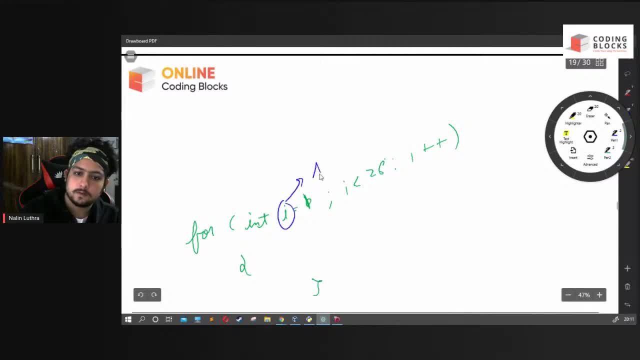 this. i here as- and we're good to go right, that's right one, and can be only as big as 26, so let's also say: equal to us. that will be much okay. what about special characters? that's right, but that's I don't know. let me check Ichabod. I don't know what that means. call your. 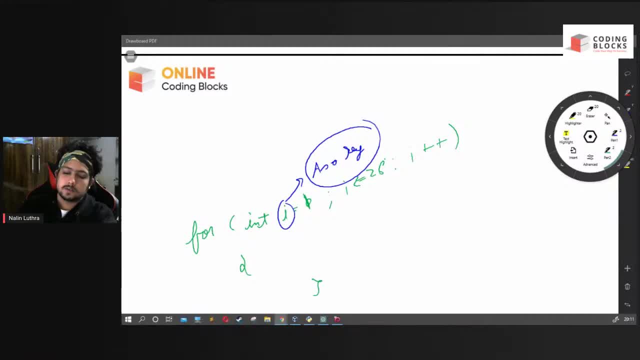 that's right, but that's a different one. that's a different one. that's like a depends on how we made the csi, for csi work was originally not made for the special characters to be taken into account. it was made for the springboard strings. also, we are not actually 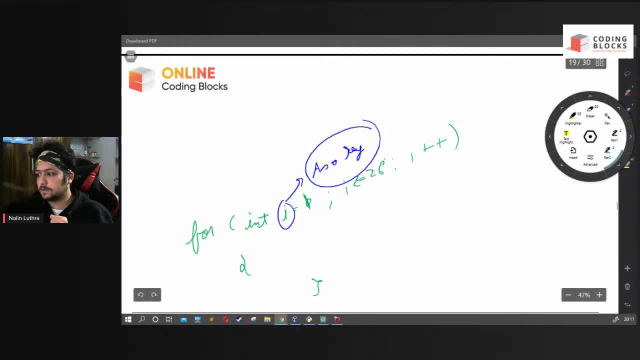 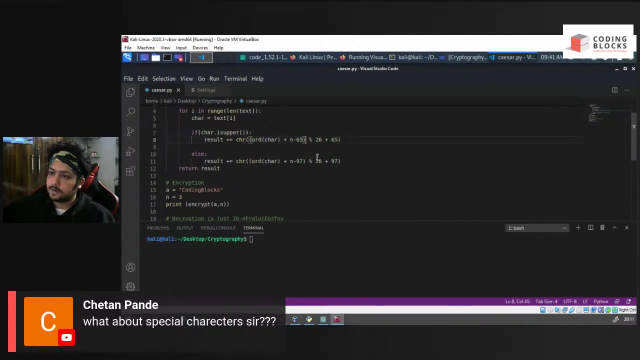 encoding those special characters. let's look in the code back itself and understand that one. okay, let's understand that one. okay, let's understand that one for now. you see, i am not using that special group for encoding. if you and i do, i don't change the value of n, right? so it makes sense what happens if i change. 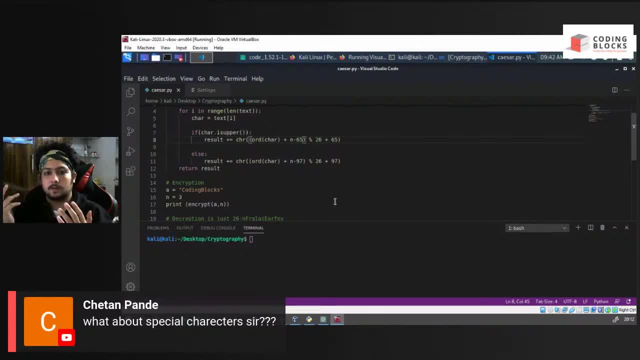 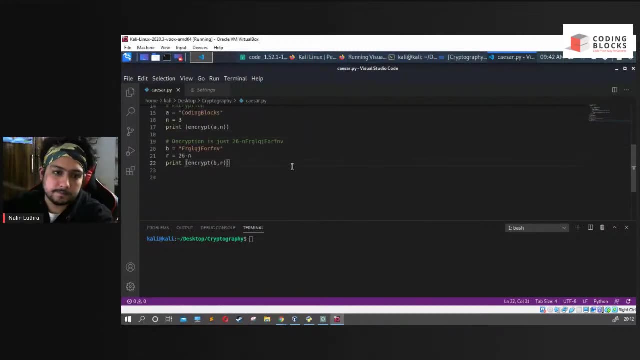 the value of n. let's say n is 27.. in that case we'll see what happens, in that case too, okay. so let's, let's try it out, let's code it, let's understand it and let's see how it goes. how big can we do it, okay? so, uh, let's comment this code all together, because 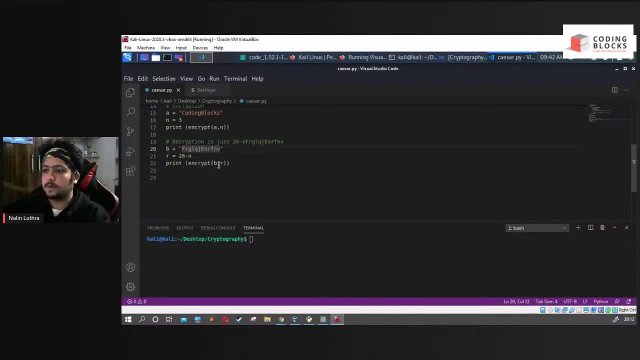 i guess you guys can see the code if you're using a laptop, if you're using a phone to view it, maybe touch. we're not able to see this. let's see if i can zoom it right, okay. so let's start. let's say: i is equal to zero, okay. and let's say 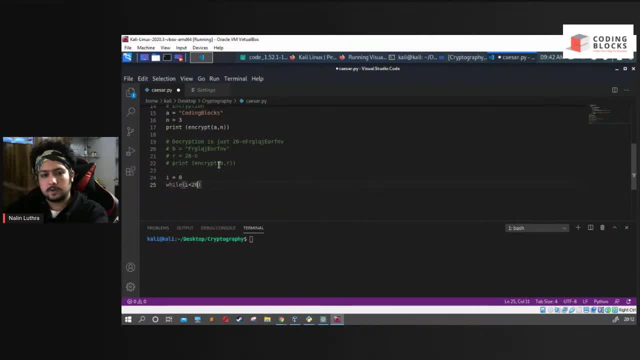 file i is less than what, let's say 26 for now. okay, uh, let's say print, uh, ok, encrypt, and the message should be what? this is the message we are getting out of it, this one, right. so let's say this, let's copy this thing. 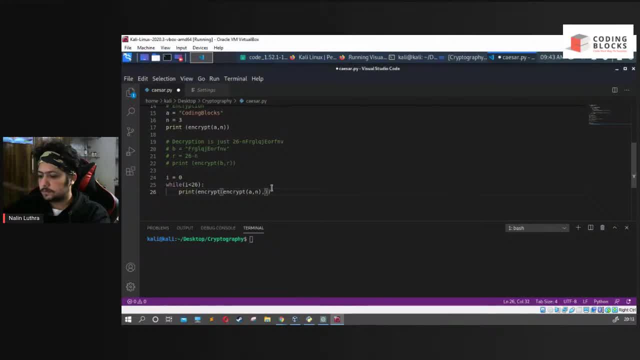 and let's paste it, okay, uh, and let's go with i, but that's what we're using over here, right, using three, and over here using this. okay, so let's have one more command print like this to a print element in python. so i don't think we need this one as well. let's see what we can. 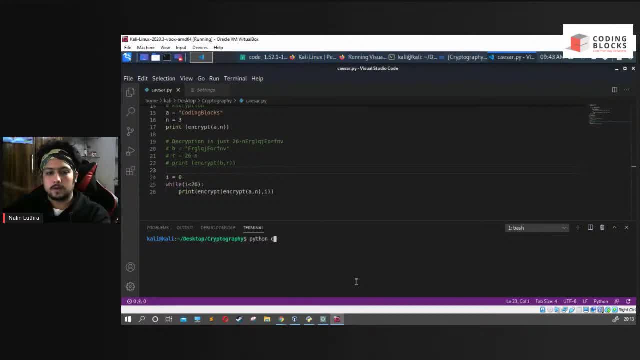 let's run the code and let me save it. let's say python to the py. okay, that's weird. sorry, i'm also supposed to be doing i equal to i plus one. yeah, makes sense, my bad. yeah, it won't hang on my system. i'm pretty sure about that. but yeah, i did a mistake. 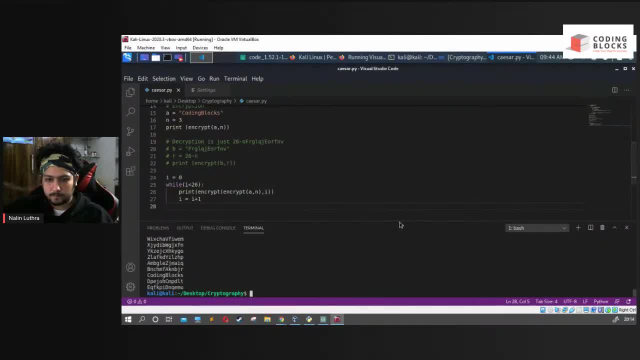 okay, so this is what i get. i get all the possible combinations for this. right, i got this, i get this everything. so what exactly do i need? so i need to check. this is the answer, right, okay, so i think, zoom. can i zoom this one? i don't know i can zoom this one or not. 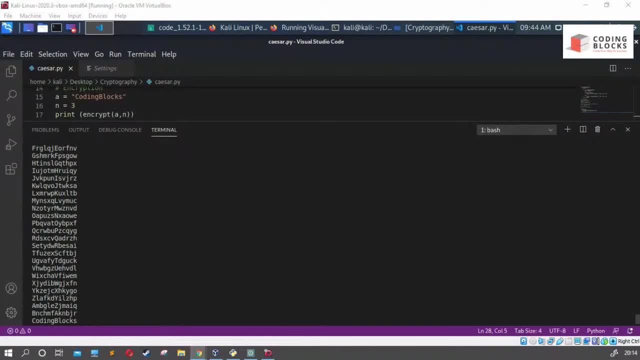 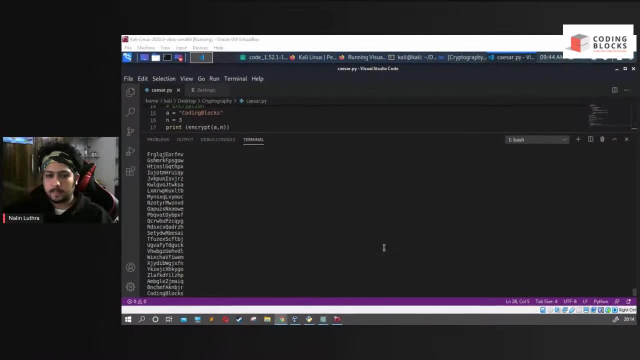 uh, okay, let me see how can i zoom. this is good, guys. can you see now? right, maybe this is better now. so yeah, you can see, i can definitely find the answer right over here. oh yeah, it's getting slow somehow. okay, my system is getting weird enough. cool, got it now you can. 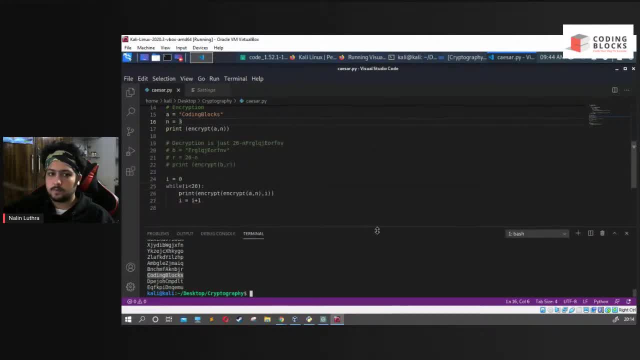 see we get coding blocks directly. so, uh, what if i just say, okay, let's print what. let's say, plus this, plus, oh, let's do that as well. okay, let's print this thing again and see what we get. somehow, why doesn't work with this? okay? 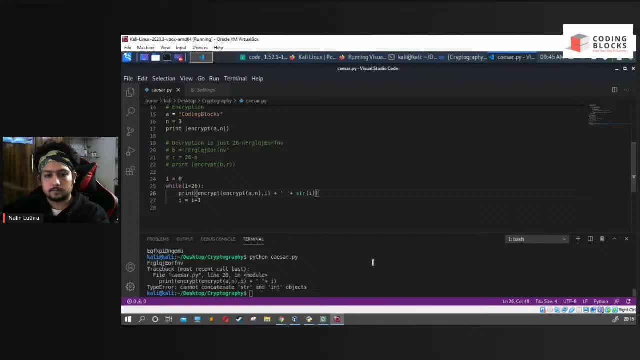 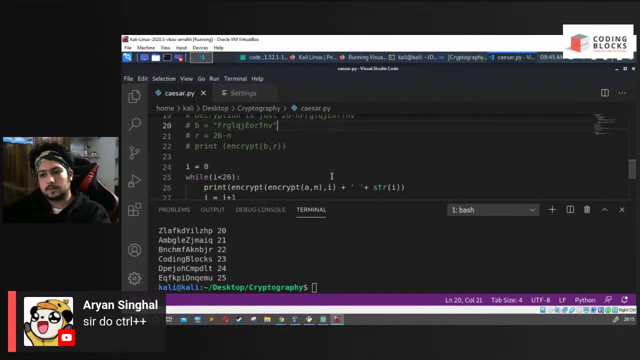 str. let's have str now, cool, okay, cool. so we got 23 right over here. we get, okay, shift and control plus plus. and okay, yeah, control plus is good. thanks, rn. control plus plus looks good. yeah, is it good now? it's weird for me now, but it will be fine for you guys, so let me just say: 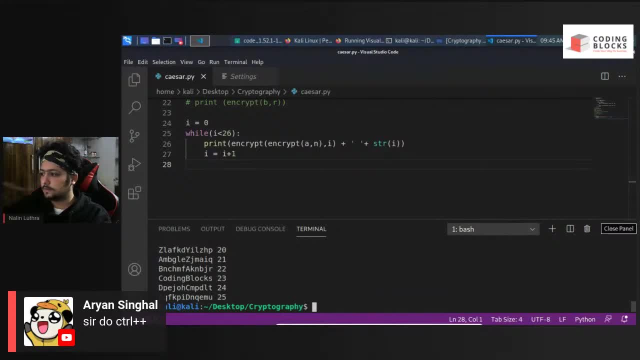 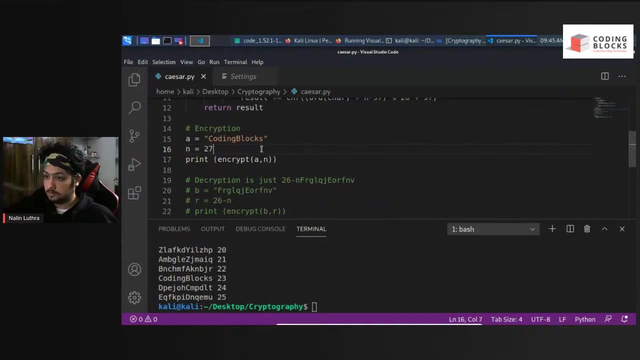 cool, all right, you guys can see this now clearly and properly. cool, okay, so, uh, so this is how you can simply do it. for example, let's let's take one more example. let's say value is 27, now that's more than 26. so what would happen? 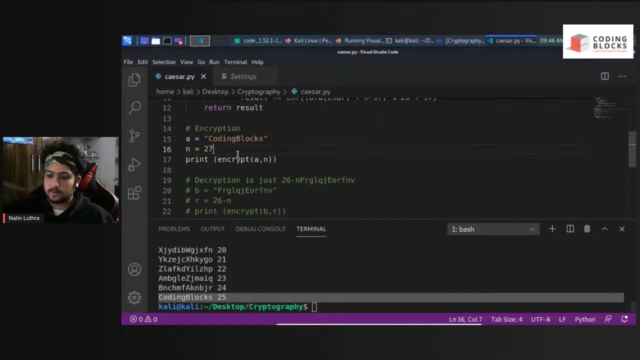 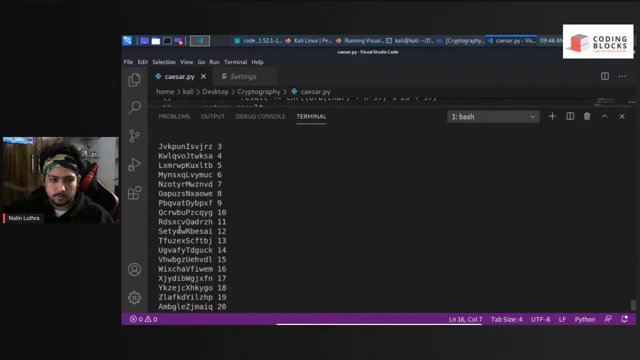 you see, coding box still comes. what if value is 30? right, let's go with 30 now and let's start. where is coding box? it should be somewhere there. it should be. it should be. i don't know should be here or should not be here. that's the question now. 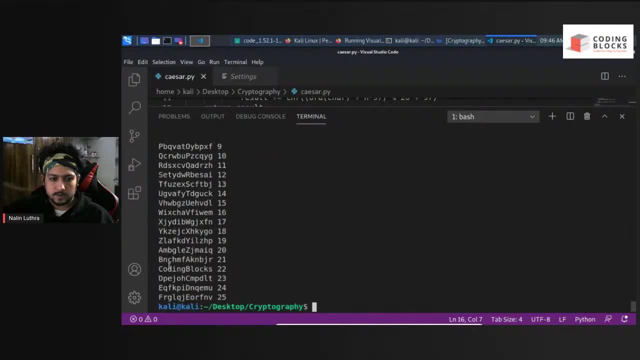 i cannot see it. okay, yeah, 32. here it is like: every time you try it out it works. it doesn't matter what's the value of n. even if n was way too hard, it will be here. let's go with a bigger number. four, let's go with 100. let's take 100 and check it out. 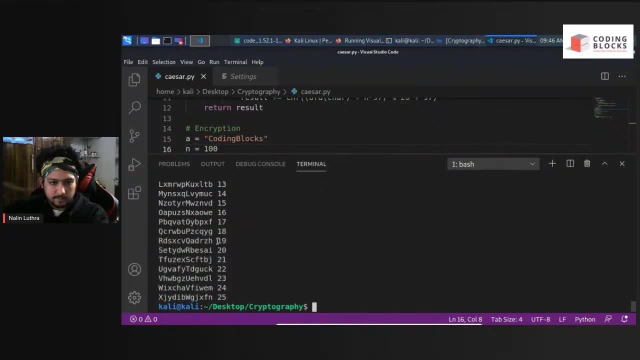 cool. now even i don't know where it is. i've taken a really big number. i hope i'm not wrong. yeah, i'm not wrong. i'm cheating somehow. why am i? i'm not, everyone know what this so okay. so we got this right. so we got on four. so that's how you actually crack a serious cipher. 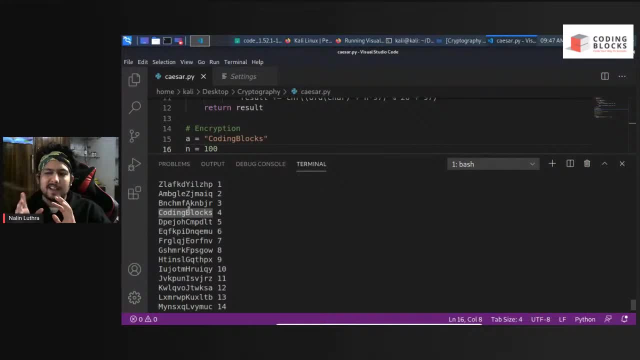 so now, wherever you see a csi- for you can guess what word should be there, and it will happen, that's right. which one? which will start repeating its self because of rotational c cipher? that's how it rotates. okay, so i don't know, python. that's why i can't be able to understand what to do. 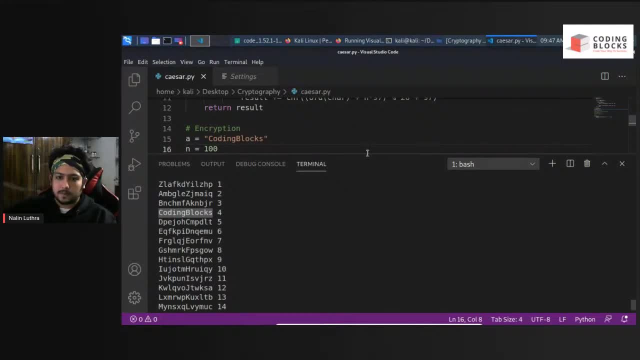 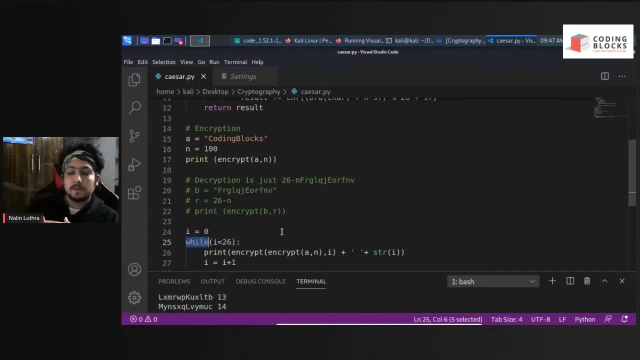 uh, python is kind of a simple okay, so what i'm doing here is just using words, right? so let's say while, while basically it's a loop, so if you're filling up with c plus, plus. that's why, if you're familiar with- uh, what language? let's take a language for now. what language is similar with? 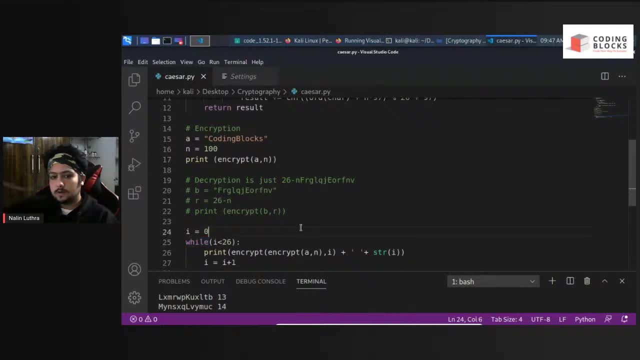 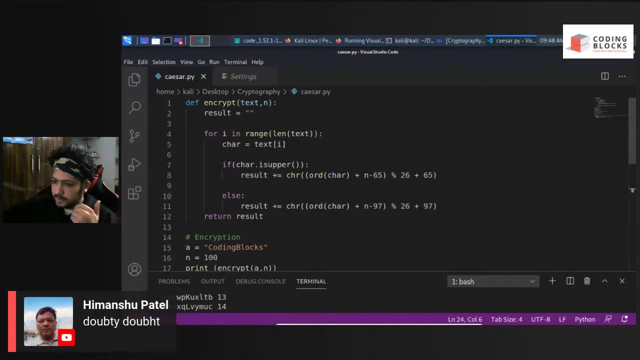 java, it's, it should be anti and so on. right, so either ways, it's fine, it's fine. so that's how it goes, okay, uh, if you got a cloud, just message the doubt in the chat. don't say though, like that's weird, i don't know what doubt you have. if you tell me the doubt, i'll, i'll give the answer, right. 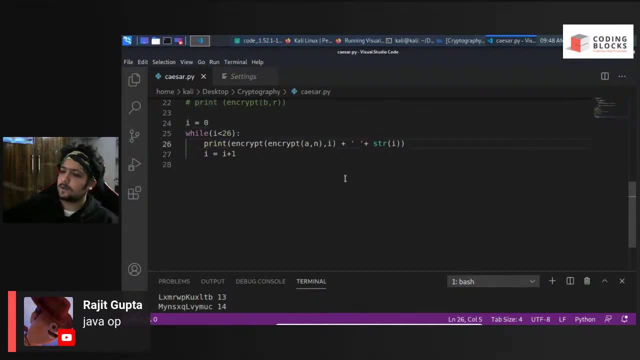 java. it's fine. that same, i think this code will work. anything you have to change in java is like this, so you would just like, since thewal synonyms of subjava's code, we have to simplify them: system dot, dot print. that's, that's what you do in java. okay, and you here, you will write end. 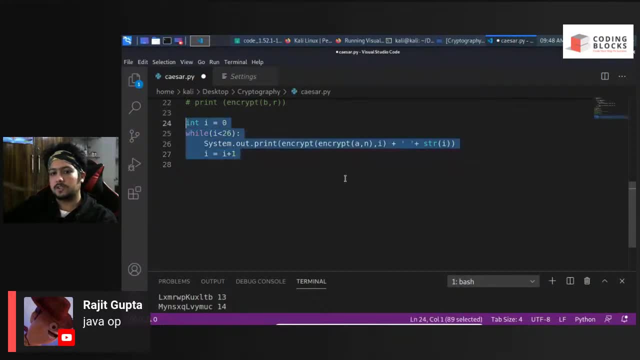 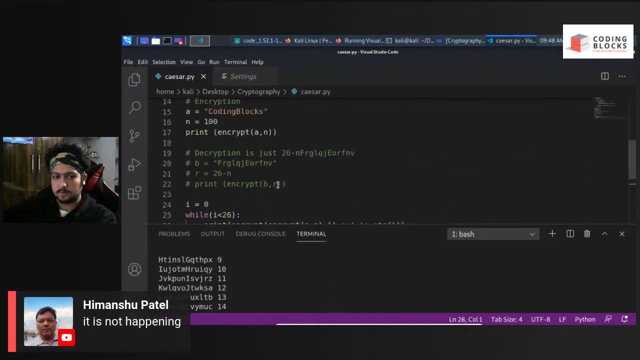 yeah, it's a java code now. okay, so this code will work in java. that's all, that's simple, okay, okay, coming back to this here, it is back, okay. uh, this is not happening. what is not happening, i don't know. uh, it's working fine. actually, you can see this code. it's working fine. see it's. this is. 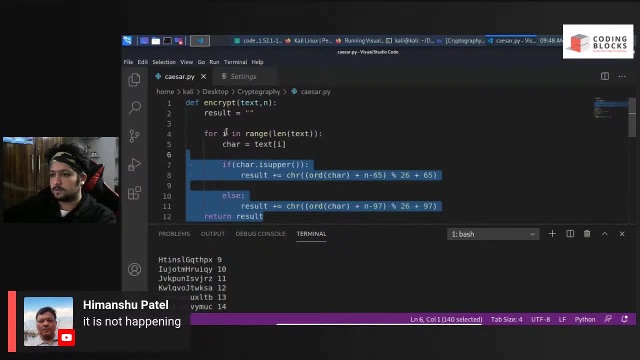 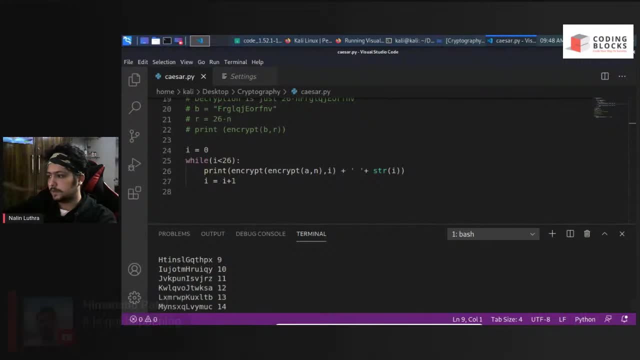 how it is. it is working fine. if you guys want to call, i will give you the code. that's not a problem, but i'm pretty sure it's working fine. i know it's working fine because it's working right now okay, so i don't know what's not happening. 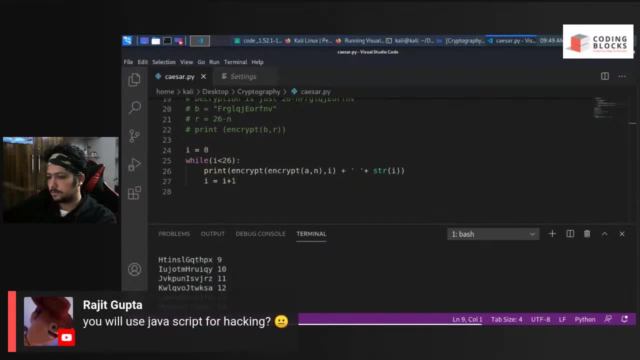 uh, okay, javascript here. i was going to school. yeah, how will you javascript as well, like, what do you want me to do? do you want me? yeah, that would be this index error. you have to write this. now. that's fine as well. you're checking me, i don't know stuff, or what. like that's fine, now, this is more. 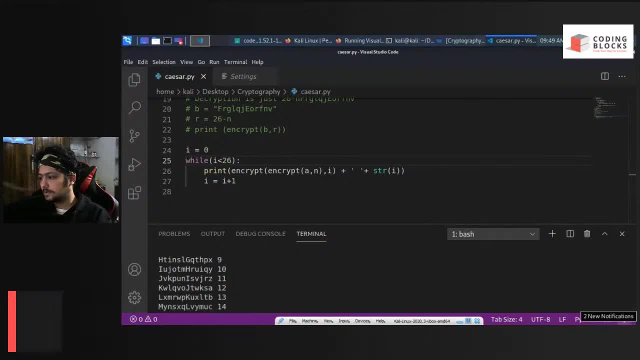 of a logic building. right, it's not about coding. i have no idea, man. what are you saying? what's not typing and what's not getting it done? i don't know, and so i i can't actually answer everything. okay, guys? sorry, let's move forward, guys, let's move forward. okay, now to 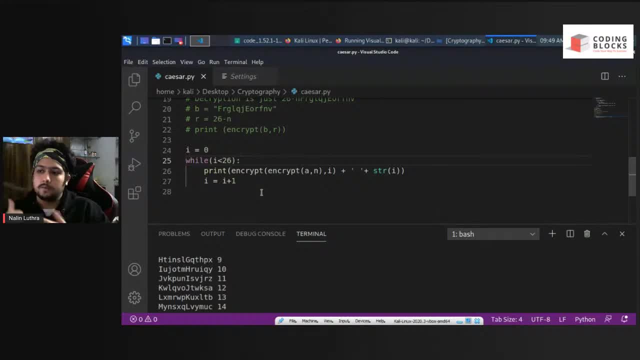 a little. look at one more. uh, cypher, we are good with csi for now. right, everyone is good with the. a cipher, we have the code, we've made a code on our own and we're good with it. uh, there is no javascript. there is javascript first of all, guys. uh, that's how it is okay. 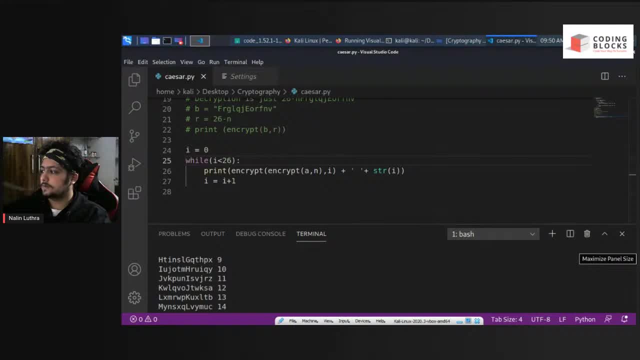 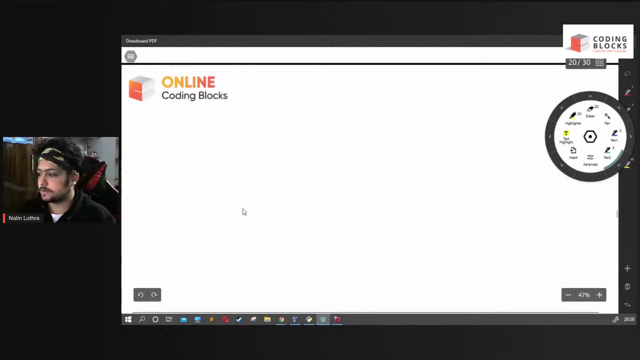 anyway, let's move forward and work towards a new cipher which is called a substitution cycle, a mono substitution site. let's build, let's see how it works. oh no, okay, here we are now. let's talk about mono substitution cipher. let's have a. get the next language work on alexa. drum roll, please. sorry. 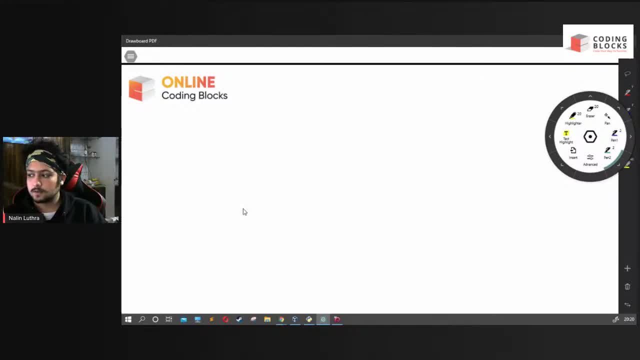 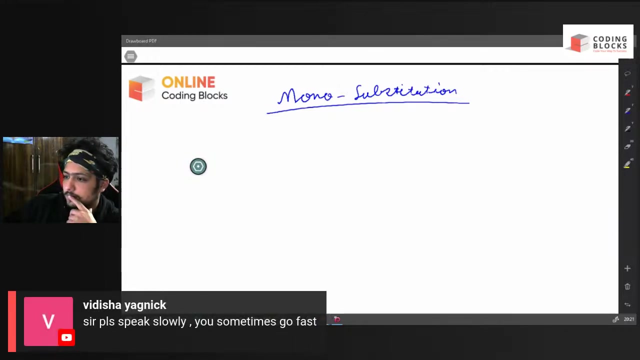 alexa: drum roll please. okay, cool. so let's go with next cipher with us. that's mono substitution cipher, okay, okay, yeah, cool. so let's say mono substitution cipher, yeah, okay, okay. uh, i will try to speak slowly. i don't know. alexa is opening, right. 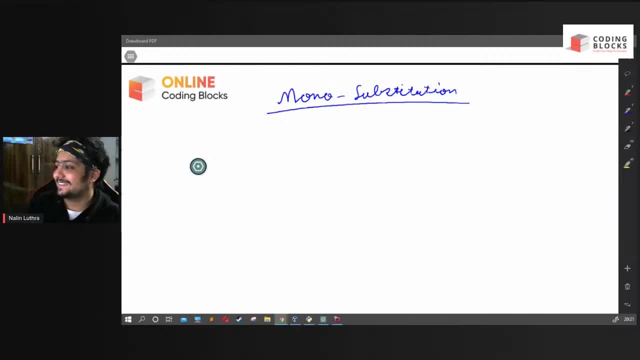 it happens a lot of times with me. okay, the links are going wrong, that's why. okay, so let's, let's speak slowly now for a while, okay, guys. uh, let's get to point now. uh, what is mono substitution cipher? so today, we have not today. yesterday we have talked about with cipher. we talked about 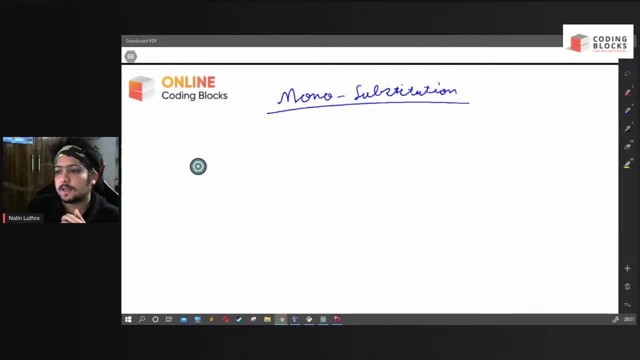 Caesar cycle. Now, what exactly is monosubstitution? So what happens in case of monosubstitution is we don't have a proper rotation right. so in case of Caesar, we used to have a rotation right. so, for example, start from ABC. okay, so we have this right. so that's how you map together things, right? so 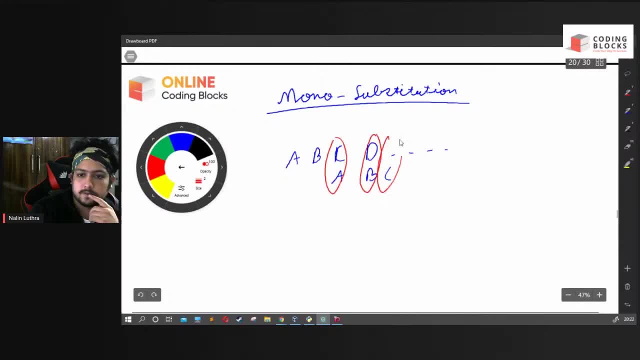 this thing just wrap like this, it's wrapped like this and so on. okay, that's how it goes. but in case of monosubstitution, that's how it works. so what happens in case of monosubstitution? let's look at that for a while. okay, let's rub it off. yeah, cool. so in case of monosubstitution, cipher what works. 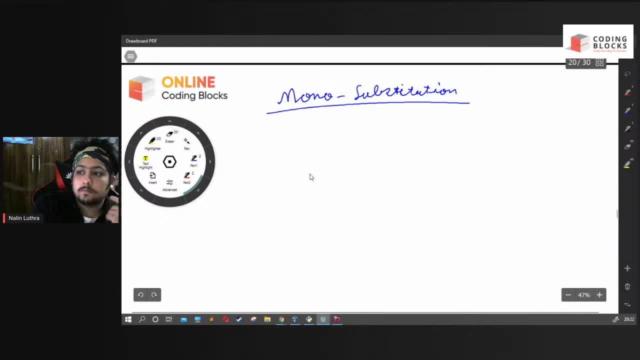 exactly? and how forward is? we map things randomly right, so there is nothing as a proper way to get it done. it's completely random. for example, let's say A is mapped with C and D is mapped with A, and E is mapped with K and K is mapped with what? D? no, yeah, D sounds good and L is mapped with I, or whatever. 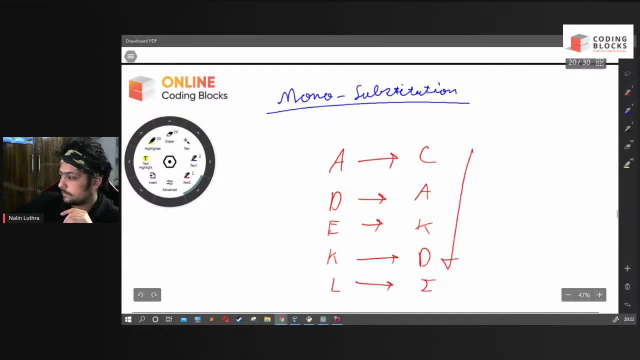 you want. okay, so that's extremely and completely random. okay, so that's how you work with the monosubstitution cipher, where you make completely random things you want to do. right? so that's how it works. is everyone good with it? is everyone good with? like did everyone? 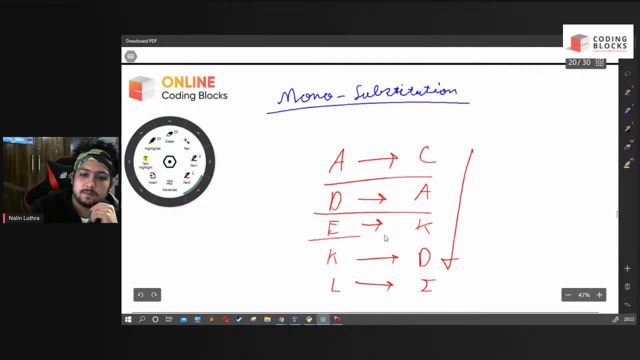 understand what is monosubstitution. we change things randomly, one by one. we change this, we change that here, there and everywhere, right, okay, uh, did everyone got it like? what is monosubstitution basically means? mono means substitution means change, so monosubstitution means changing one right. 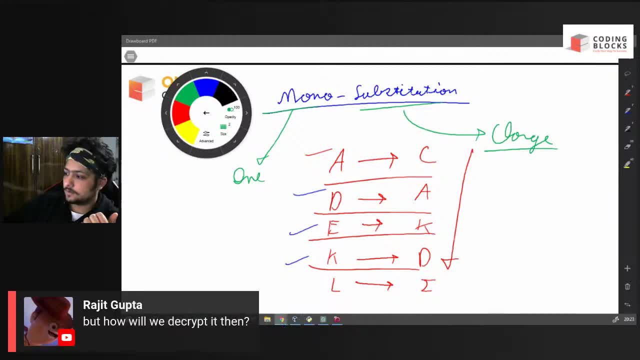 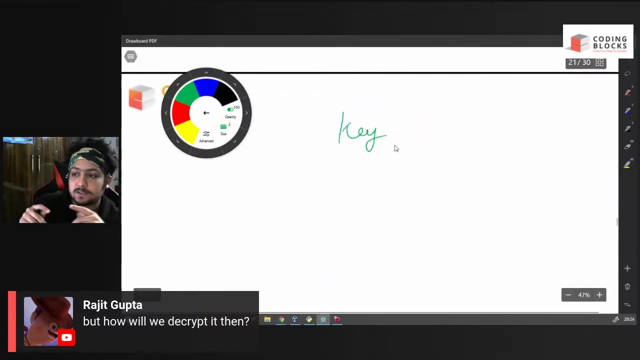 not really part. if you don't know the algorithms, you wouldn't be able to decode it. so yeah, it's kind of like slightly different because we know the key right. so what happens is you know a key. in case of Caesar cipher we had, we can actually guess a key because key is supposed. 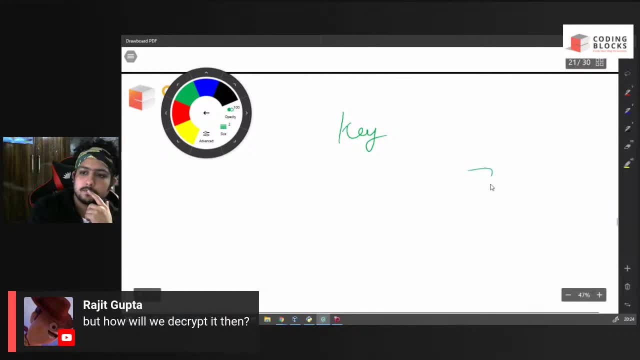 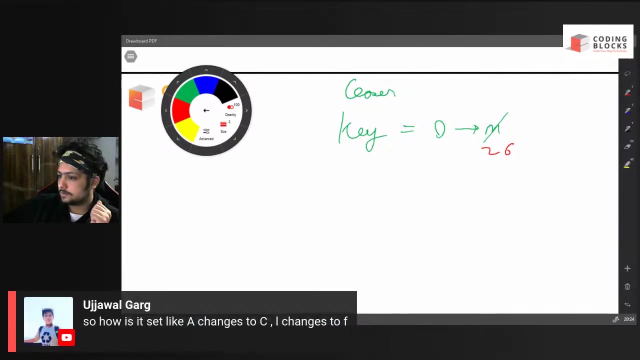 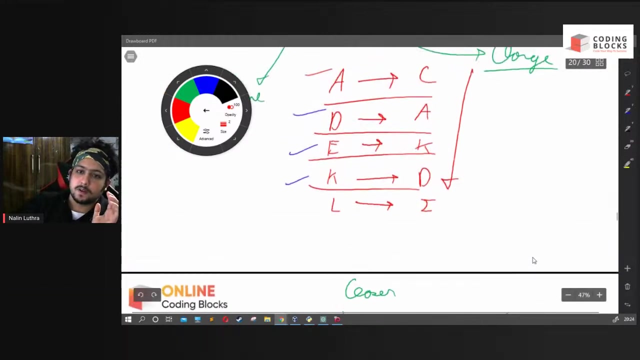 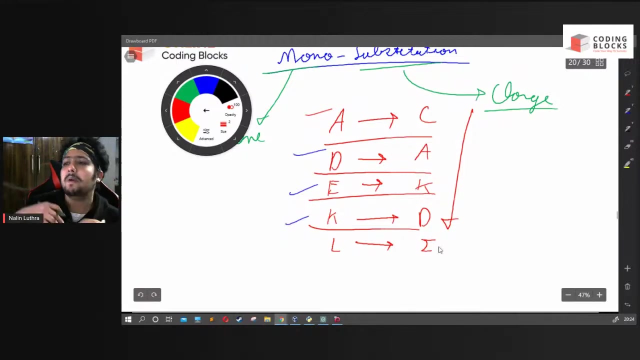 to be limited range, right? yeah, cool, it's got to work some more time, okay. so key, in case of Caesar, cipher key was in range from zero to n and n over here is 26, right, okay, right, would you go ready? right, it's random, but but 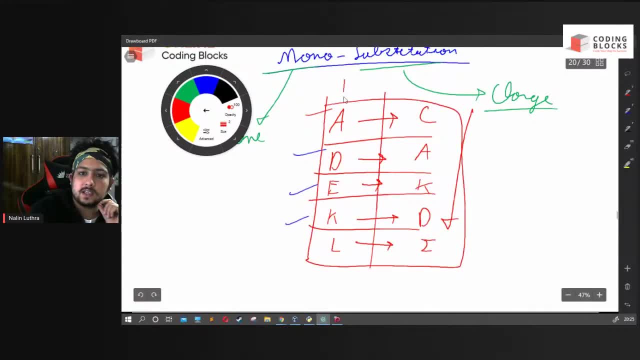 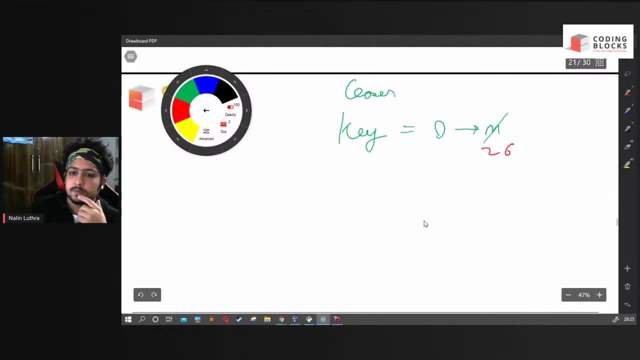 um, now cheese, you put it in here, are you getting it? so Caesar, cipher, a case may keep Nick, he's possible thing. 0 to 26, but but it's the case may get nice key possible, right? actually it's like 26 into 26, that's dance, that's how many. 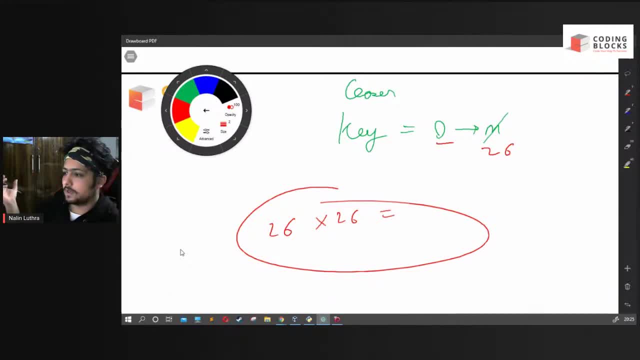 keys. am I from wrong? let me know. I don't know if I want to pair 26 alphabets with 26 other alphabets. how many possible scenarios are there? that's simple. like to change success for truth, right? that's what I think. believe me. 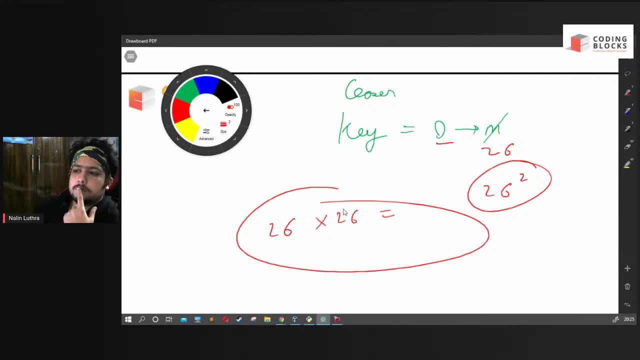 that everyone has to have one. I'm wrong. I don't know. maybe I'm wrong with probabilities. I don't know, I have to check it out, but I think it will. okay. I'm a point: is it's a big number? that's the whole point, right? no, no, no, no, no, no. 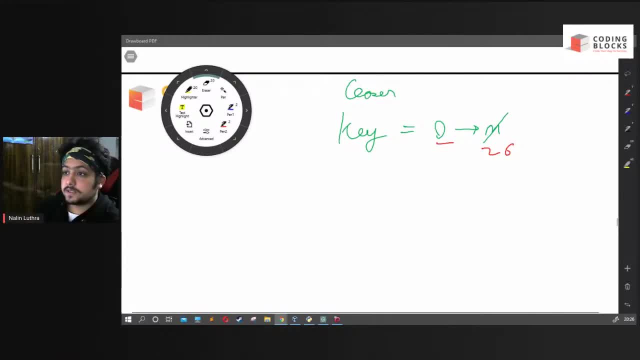 no, 26 are not there, it's, it's more than 26, because let's say a. okay, let's talk about a. so a can be linked with B, C, D, E, F, G, anything from 26, right? a can be linked with anything from 26. let's all be so. B can only be linked with numbers. 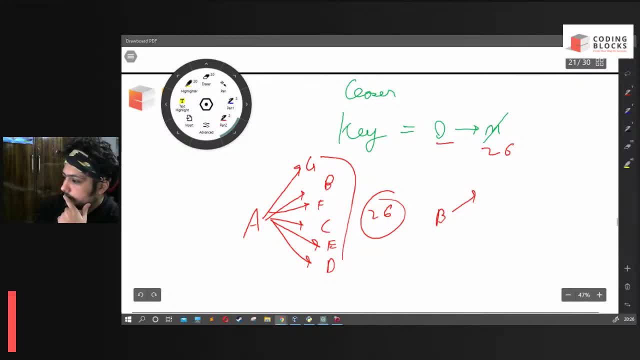 which are not there right. well, maybe I'm wrong with 26. that's not the right answer, maybe I don't know. I'm not sure about that, but it's a big number, it's a. n is a big number and it's not easy to cut. so it's about B now. so B can be linked with what? anything except. 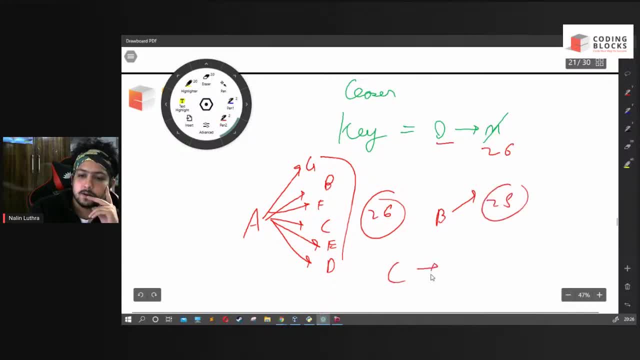 for 26 is. so we got like 25. see, you got like 24 and so on. so we would have 26 into 25, into 24 and so on, like that's how it's okay. so my answer is wrong. so you have, how many keys for this one? I'm wrong with 26. that's not the right answer. 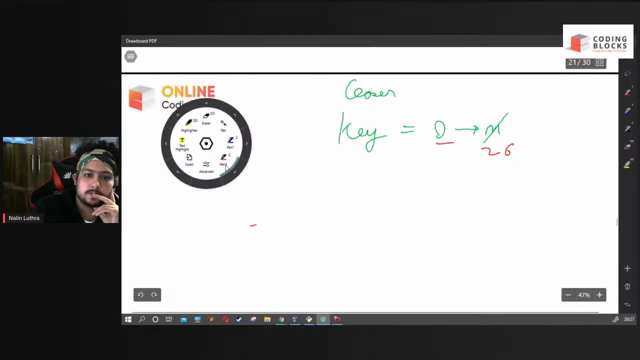 I told you how many keys are there. it's so simple. we have what 26 minus 25 into 24, into 23, into ready 2, into 21, into 20, into 19, and so on, up till 1. yeah, that's how it is. so it's like: okay, let's, let's make it by 26. back to you, these many. 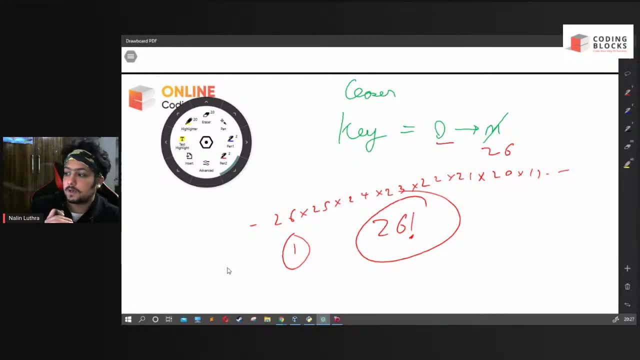 scheme are required, right? yeah, so that's how it's working, right? so maybe I'm again, I'm wrong, I don't know. but point is: it got many keys and that's how it works. okay, that's my point I want to make. I don't want to make a point. keep. 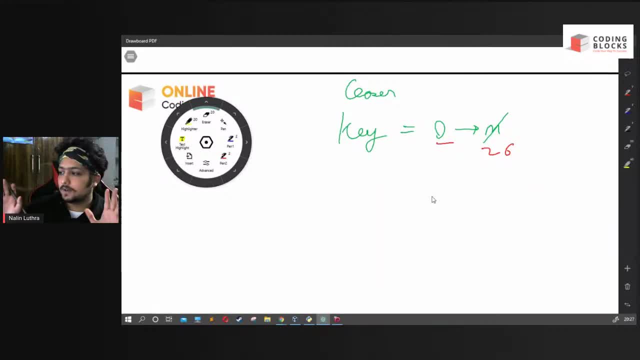 together. I know the answers. I'm not good at maths. I'm great at maths. I don't know, but yeah, it's a good point, it's a good thing we got many keys all together and we won't do it. so in that case n becomes large and it's become difficult for. 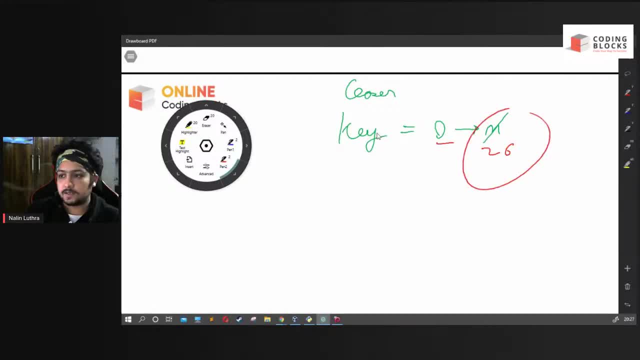 anyone to crack the key all together. am I right or am I right? I'm right, okay, so I'm not sure it's right or wrong, but someone else answer over here. maybe it's right, maybe it's wrong, yeah, so we got big numbers over here, right? so, uh, so, 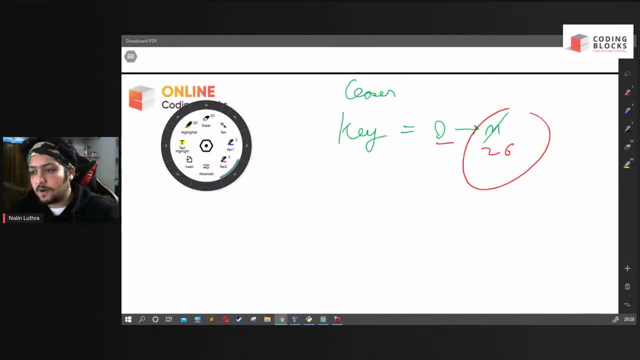 that's, that's the point. so let's move forward and let's write the code for substitution cipher. okay, that's weird. I think I should have a voiceover like thing. right, they were all substitutions like mono substitutions like boom boom, boom, boom, boom boom. that would be cool. I'll figure it out somewhere, right, not like cool, okay. I. 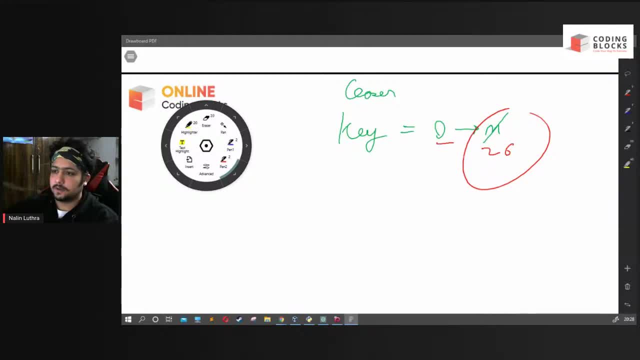 don't know. okay, people are like fighting over this monster market, cash or mafia and whatever not. let's see, let's do it. why I'm doing it? I'm not doing it over here. I'll write a code for it. if I want to, I can write a code for okay, so let's. 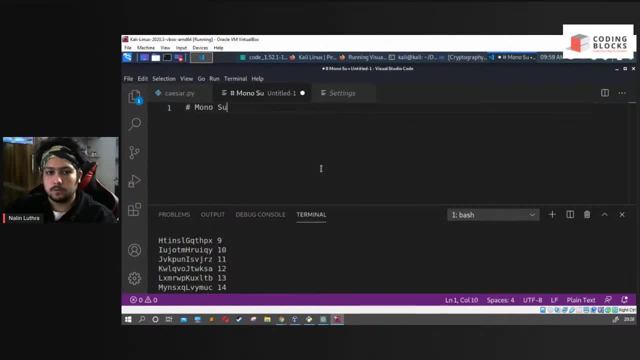 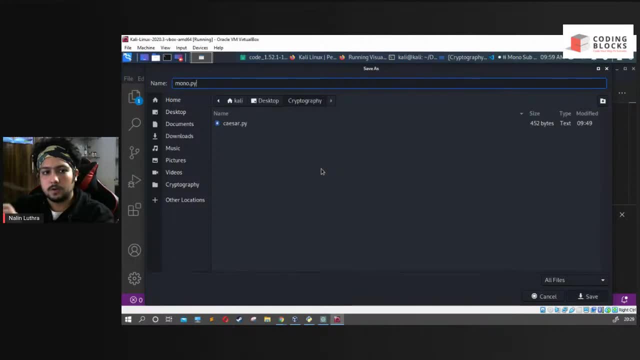 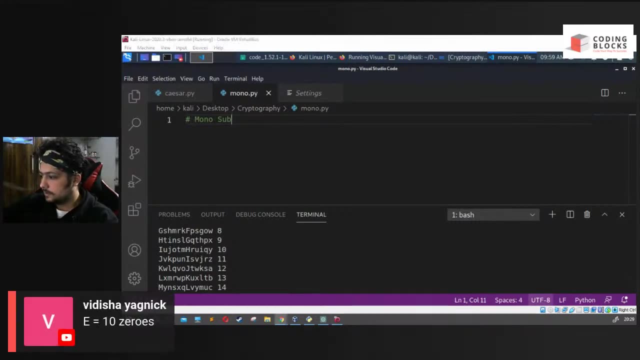 move forward and work with monos substitution. so okay, let's call it mono dot py code: monos substitution. let's work with that one. now. I got many messages. yeah, that's right, Sushant, I can make a little track for something like something like this: right, that would be cool, okay, anyhow. 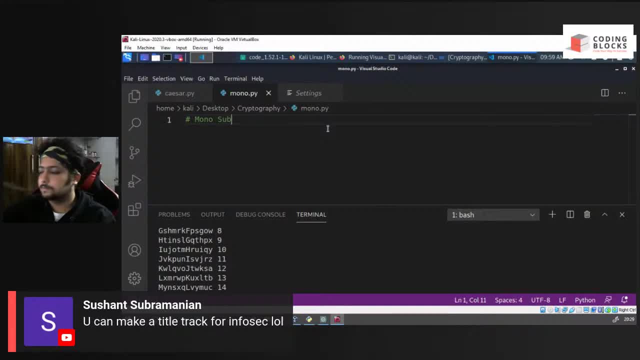 until, unless we make that track, let's just say dum dum, dum dum, sorry. okay, let's say monosubstitution. I'm bad in friends, sociability, I don't know what. I'm good. sometimes I feel like what's happening it on the world. we are really slow. let's move forward. 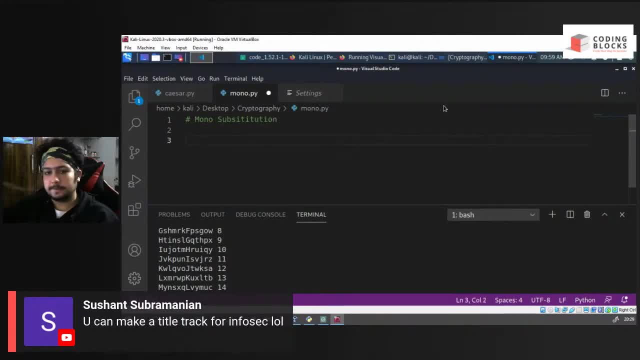 monosubstitution. okay, that's right. okay, well, why are we having a discussion on what's right and what's wrong in this case? let's move forward and right. the core itself is rather cooler and nice and fast and better way to actually learn cipher. where do we load these items? okay, I don't know. let's move forward. and talk about that later. er typical recursive voting risks examples. alright, so we're just going to work on the code itself. okay, that would be cool. everyone will like the code if we. we don't love this video a lot, but like attend to it. thank you so much. I hope that was a good 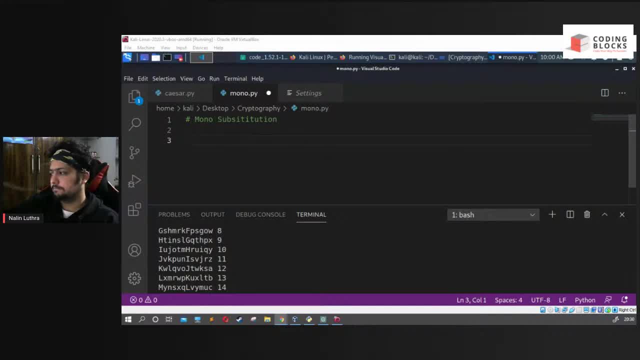 things. so, first of all, let's make a key. okay, i did make a key previously. uh, let's, let's make a key first of all. so the key is equal to. so it's not typing. it should have been typed over here. okay, uh, i got something over here. yeah, good things are set. now let's go. so the key is equal to. 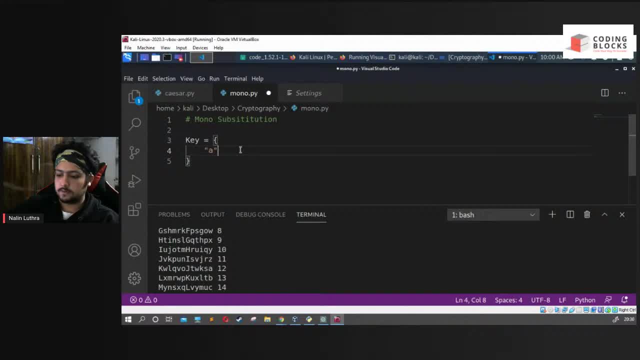 let's start the key. let's start with a right. okay, let's start with a. okay, let's say with z. okay, let's start with b. this is boring man, i will like took me a day over- like seriously, that's a long time- to get it done. 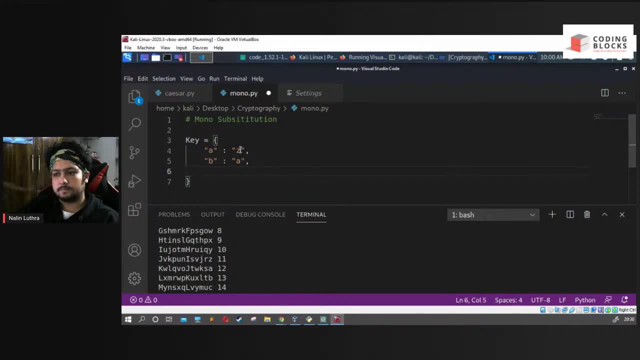 let's go with c. i don't know, it's weird. should i do this one? should i code for generator key, something like that? that's a weird way to do it. what took me so long, took me so much time to actually get this thing done? it's like a, b, like. 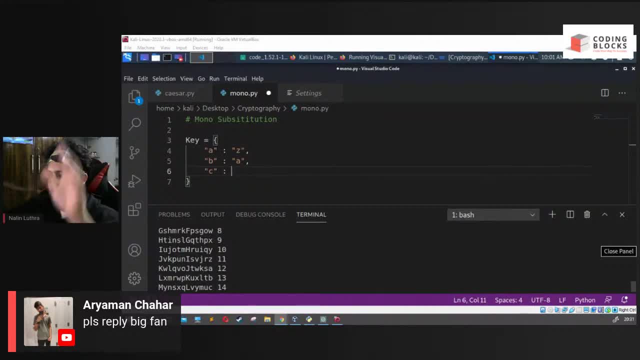 hey, aramon shattu. what's up like? hey, okay, my spelling is wrong. like this substitution: yeah, okay, cool, right, so let's go forward now. actually, it will take me a day time to actually make the key, so i will just copy what you already have. i have made a code previously. let me find this one and yeah, let's go. 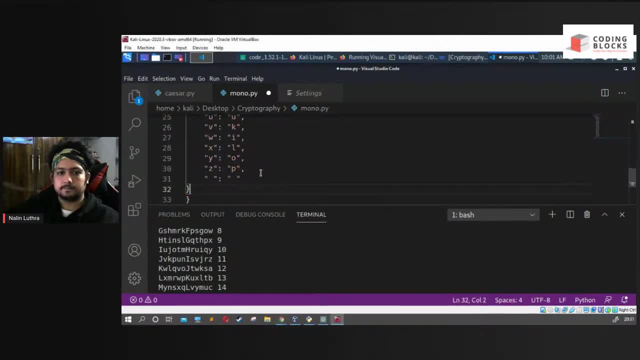 okay. so let's say like this: cool, i have you already with me, let's take this one. okay, i will share the key with you guys. that's fine, i already made this key. let's get this thing done. so i have a key with me now. okay, so uh. 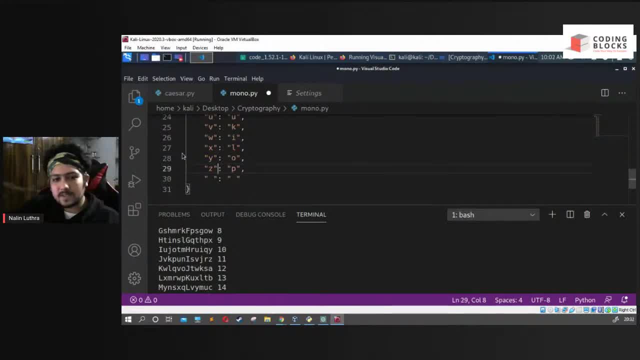 fine, like that, you just have to make a key and like, cop, like, just copy this key or make your own. i don't know. whatever you want to do, you just have to map things one to one. so that's a dictionary, right, this is a dictionary. those who don't know python, i should tell them this. 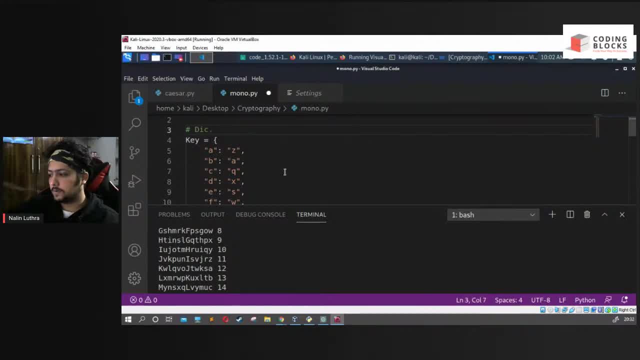 is a dictionary. okay, so this is a dictionary and that's how it works, right? so, uh, let me send you the code itself as well. okay, yeah, i'm just in the code in case, uh, someone wants it. cool code send and chat guys. so, if you want, you can get the code from the chat itself. uh, this is a. 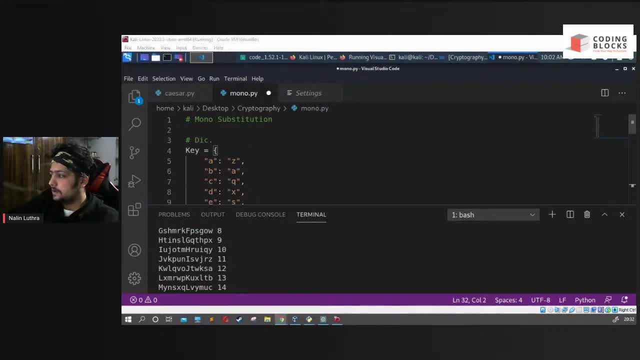 key which i made. take it and let's. let's back to this one. okay, uh, now let's try the code for encoding. that would be cool. okay, let's go down, down, down, down down. someone's not working that good and calling. i think i should code in the. 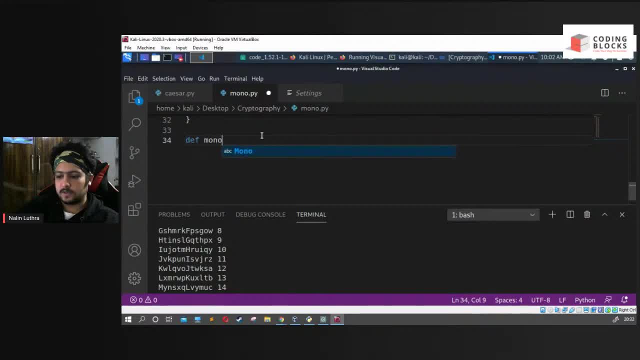 my normal windows. but whatever, let's do it. so let's say: mono and code: okay, that's how we get uh, we will give a key to it. that's important. and we also give a plain text. that's important. right, let's move forward. now we've got plain text and everything. so let's say: plain text is equal to: 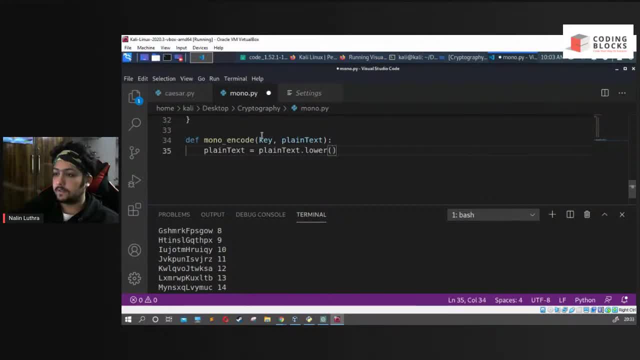 plain text dot lower. that's important because i will make everything lower. i don't want to get the complexity of handling uppercases and low cases separately. let's go. okay, now let's talk about ciphertext. okay, so let's say ciphertext is equal to nothing, because that's what we have to generate now. okay, so let's say for i in 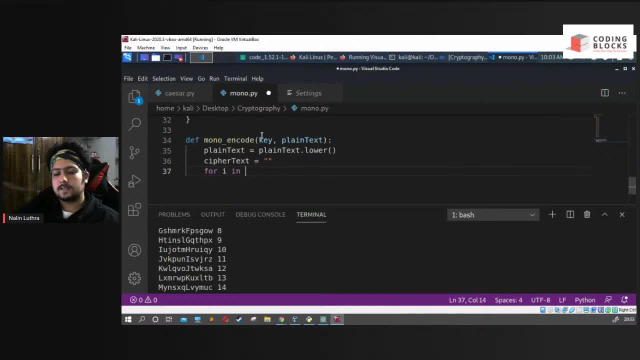 range. anyone got a doubt in the pillow? i don't think so. let's say for r in plain text. let's go to plain text and let's say that ciphertext for text is equal to ciphertext plus plain text i have over here. that's right, and we'll return what ciphertext. so what will this function do? simple. 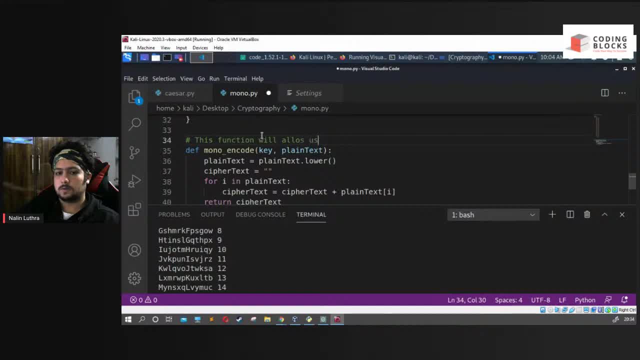 this function will allow our let's move forward. okay, i will take the account, i will do what will ask me to do. okay, let's move forward now. let's say def. now let's make something for, uh, encode, decoding as well, okay. so let's say effect decode. 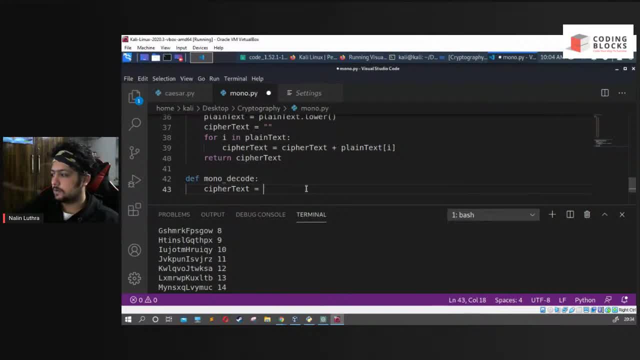 right. so let's go decode. let's call about: like ciphertext is equal to what ciphertext dot lower, okay, uh, what variable should i pass in case of decode, like i should key? that's important, right, key is important, he's like super important. i think i'm getting something wrong, where it should be keyworded as well, because, as you can, 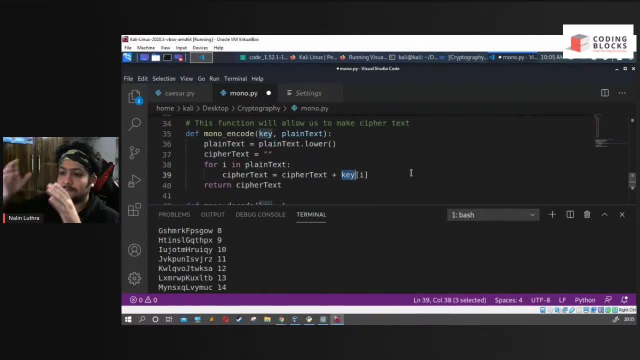 see, i'm using plain text. it should be key because that's what i'm using, right? so i'm basically mapping things. that's why i should be using key over here. right, so we call what ciphertext now? right, so fiver text. uh, now, what should we do? we? 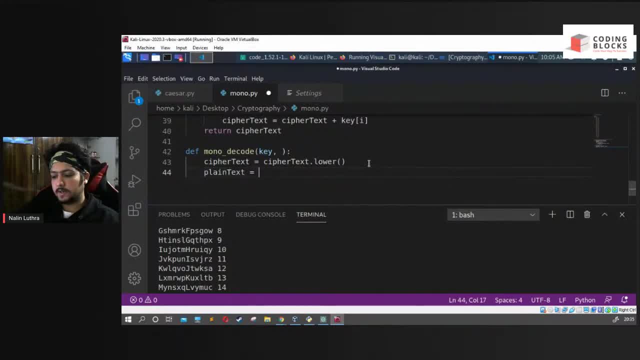 have ciphertext, what should we do? we should make a painter, right, we call it plain text, end grab. good, uh, we should also have cyph Pascal over here. let's have cyphertext and we've got plain barreaux, whatever actually up. okay, uh, really i don't know how to make my keyboard like. 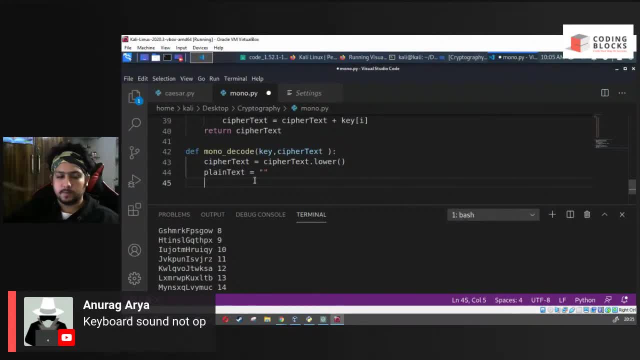 please just type slowly keyboard here. i can do that, okay. so now let's move forward, guys. so let's have, uh, okay, okay, now we have. what we have to do is we basically have to reverse the key, right, what you will have to do is it's. 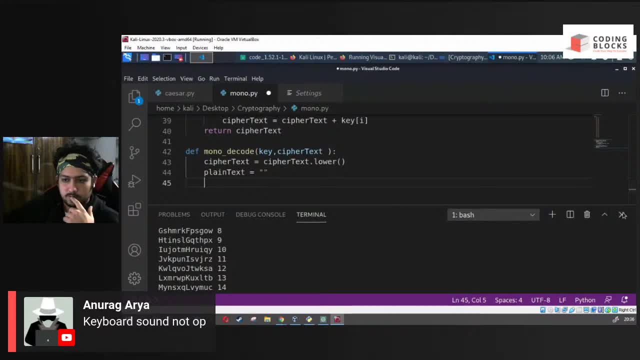 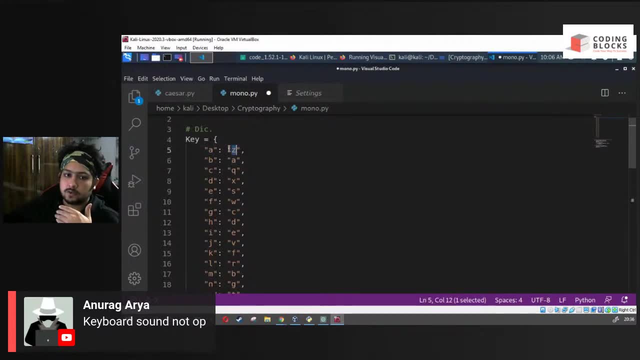 we have to reverse our dictionary. so what dictionary we made? okay, uh, we made this dictionary, right, guys? uh, we have to reverse it. now i have to say that this should come here and this should come here. there's two way to do it. point number one: uh, one way is to actually just copy. 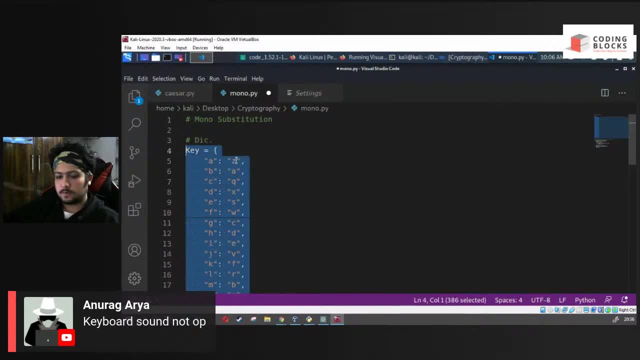 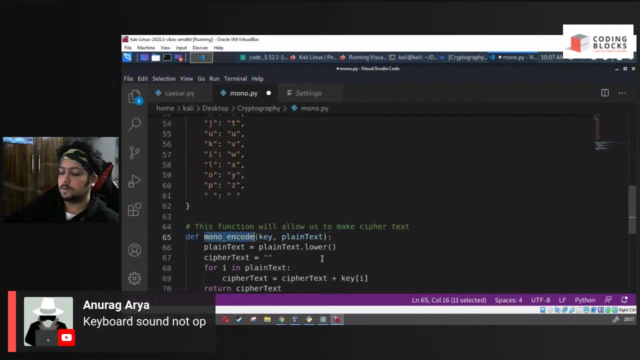 this key, copy it, make a new one over here. okay, copy this thing whole, cut it over here, delete it from here and call it decode key. that's one way it will work fine and i can just simply use the same mono encode method and with this decode key and it will work fabulous. we don't have to actually write a mono decode. 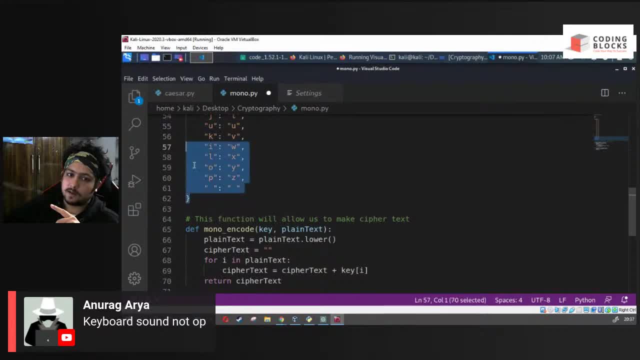 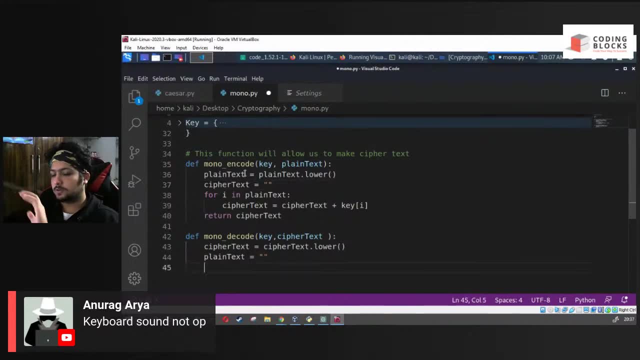 method altogether, but that's, uh way to do it. okay, we should not have two different keys. uh, because if we can work on one single key, why do we need two different keys? that would be a stupid way. so if anyone comes up with that way, uh, uh, it would be weird. okay, so what i'll do is i will make another. 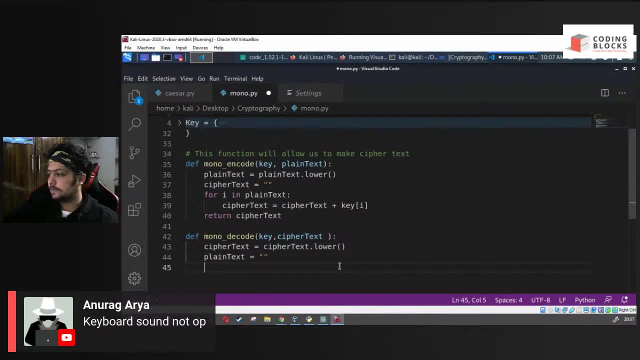 code for it. so let's have uh keys. let's have list list of. let's make list key. okay, that should be. uh, let's make a list, altogether list. okay, we have key dot keys, okay, uh. those who don't know python, again, i should tell them this: keys will give me all the values of the picture, right, okay. 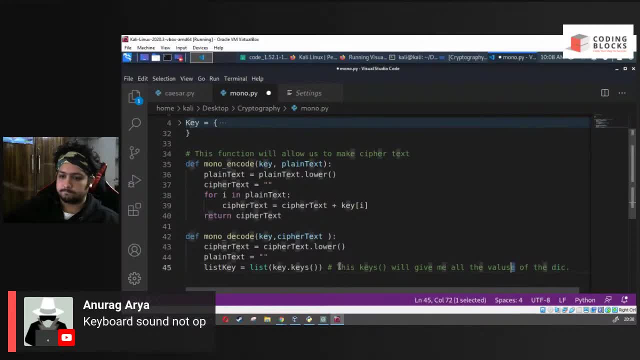 so not the value. i'm sorry. these will give me all the keys. now we have list values, right, so let's call it this value. we say list, okay. now let's say key dot values and i will have all the values with me. all right, so this will. let's copy this from here, paste it over here, okay. 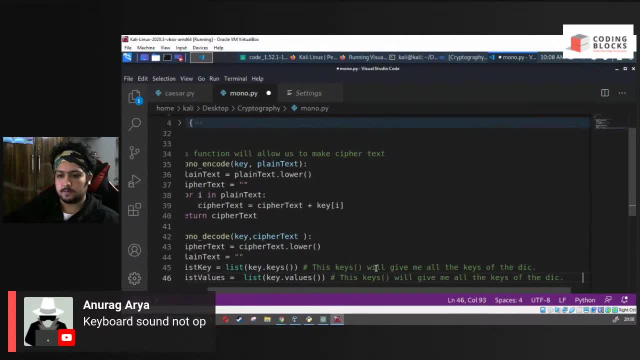 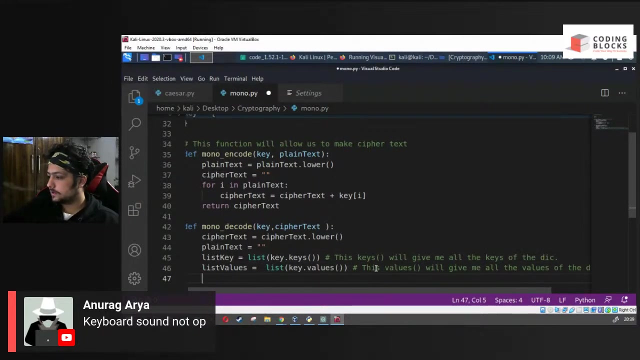 let's close it down. let's run this and paste it over here. okay, i should just call it whatever, like values, cool, oh, i don't know. some people messaging me. i don't know what to say, i don't know. okay, let's say for i in ciphertext, because that's how we want to change that. like: 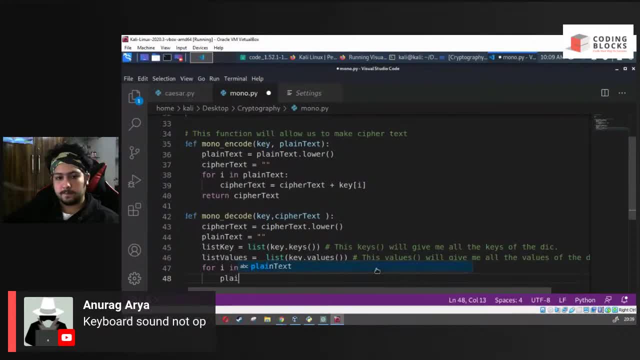 ciphertext right, so forward. uh, we say: plain text is equal to plain text. plus, you can also just shortcut over here. let's use shortcut now, so you should know how you should actually write codes, don't you know? use shortcuts. okay, what's this? what? what do i do? 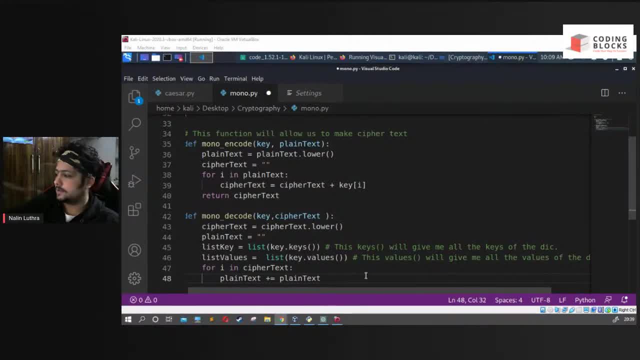 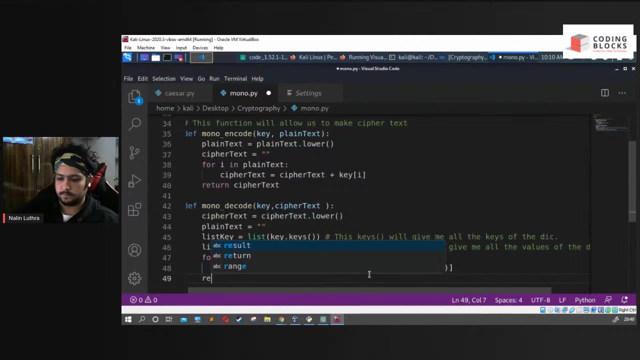 you should never be late, man, come on your time. okay, not so plain text. okay, let's have, let's have lists. okay, i will just give this values and with that i should say index and i should say i and it's done. hopefully, i don't know, we'll see. 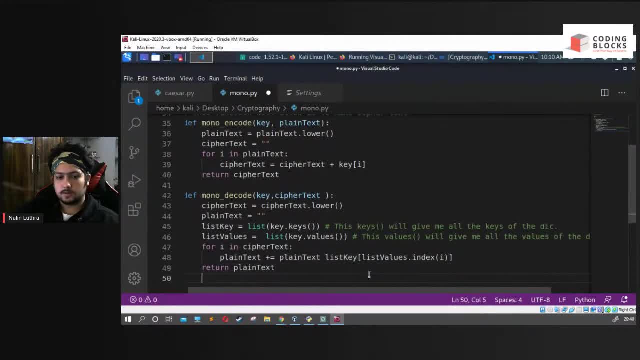 return play text. i have lists and with that i should say i should say i and it's done. hopefully- i don't know who's here- text. i think it will work. i'm not sure because i just written a code all together. let's see if it. 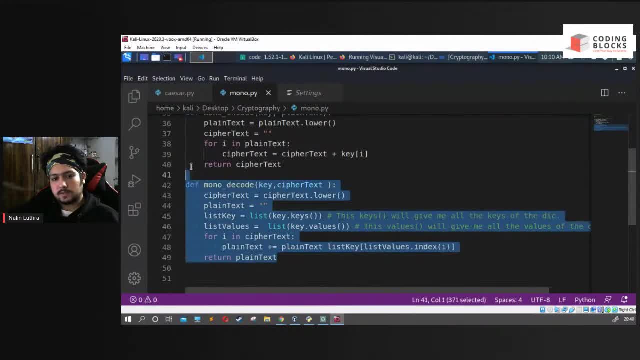 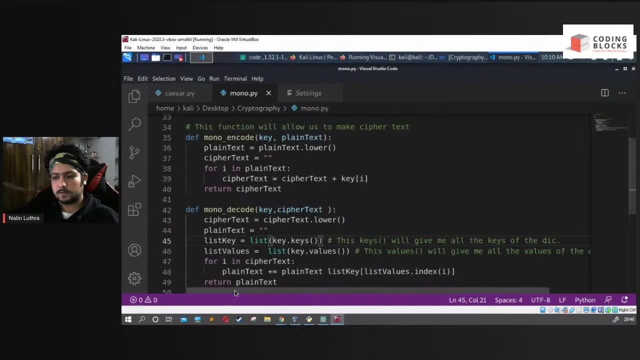 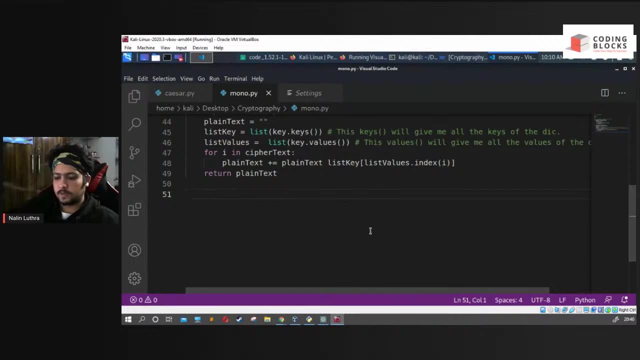 works or not. i don't know, my code never works on. first time we'll see. okay, so you have mono encode, we have mono decode and everything, okay. uh, i think it's good, it's good, right? everyone don't understand this one. let's go, it looks good to me, okay. so let's uh write something and encode it, okay so. 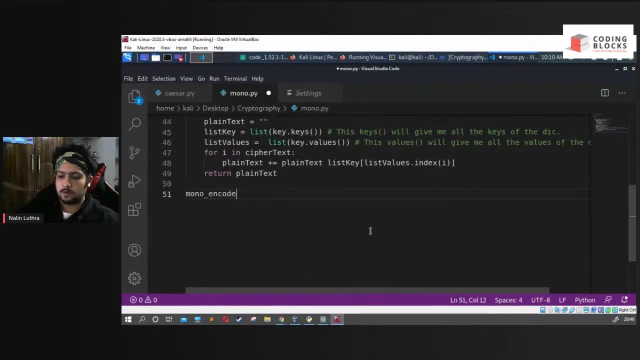 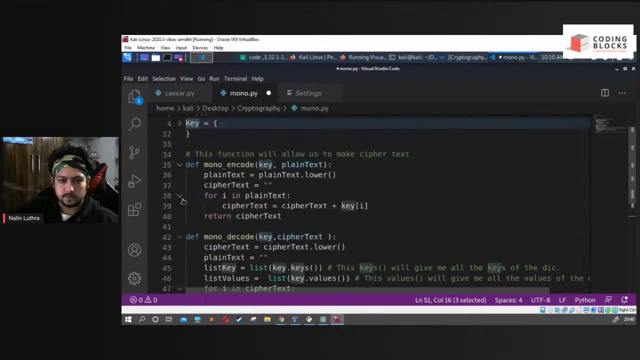 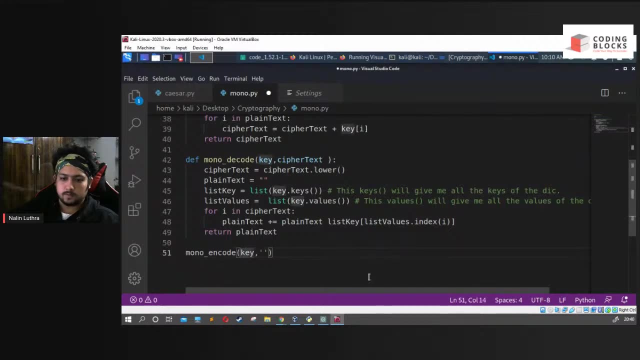 let's say: mono code, let's encode: uh, let's send the key. and what should we import? we should, i think, keys this one, this key is right. i don't know. we are using capital q, small, okay, not small. okay, overhead, small tool, yeah, cool, okay. so now let's, uh, let's what, let's put null in. 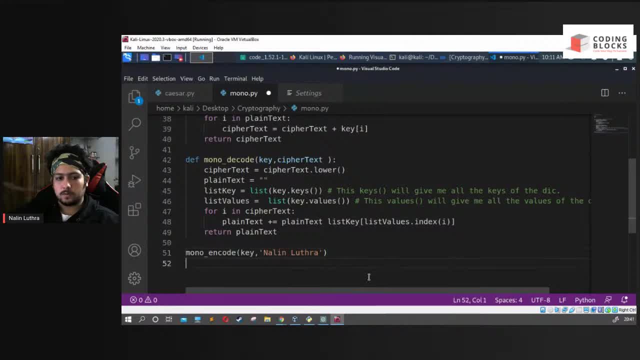 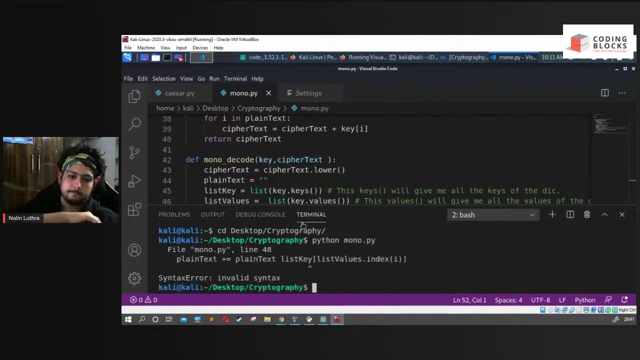 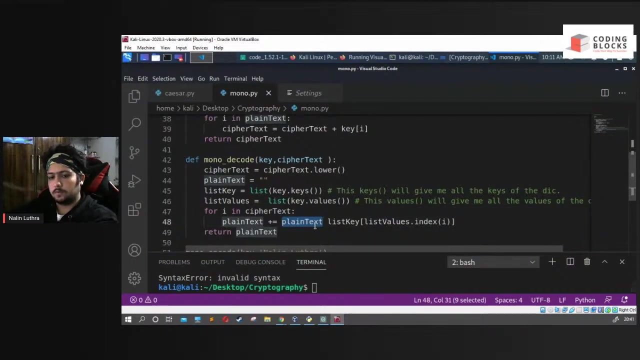 let's import this cool let's code. uh, how to do it now? let's run new terminal, let's say python monopy. okay, it's not here. i should go cd desktop slash cryptography maybe. yeah, python monopy. ah, told you, my code never works in first time. yeah, my bad, this should not be there. 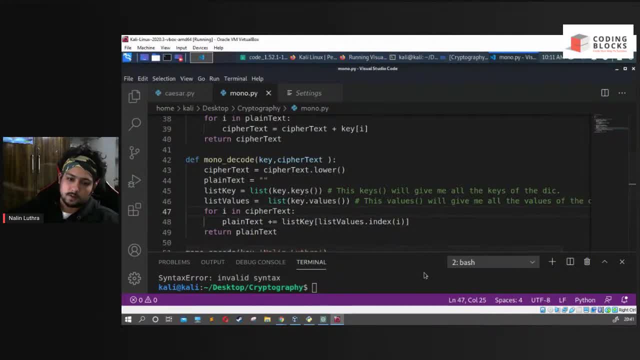 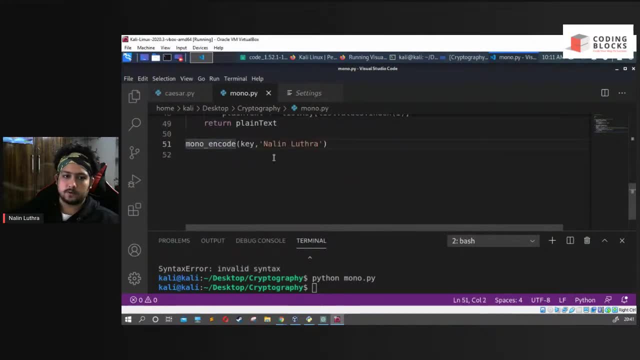 see, never, ever. anyhow, okay, let's say: or py, what we got, we got nothing. okay, because i didn't print it, i should print it. let's say: print right. actually i'm using python 2 over here, so it will work like this. if you're using python 3, uh, you just write this, that's all. okay, this is real quick, so i will. 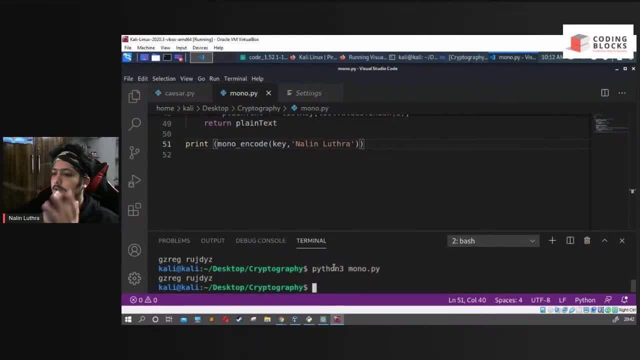 say like python 3 monopy. yeah, see, it works fine. so either way, it should be fine. okay, now let's see how to decode it. okay, let's copy this thing over here from here. why, okay, cool. let's say let's comment this one. right, let's say print mono decode: right, we'll call it okay. 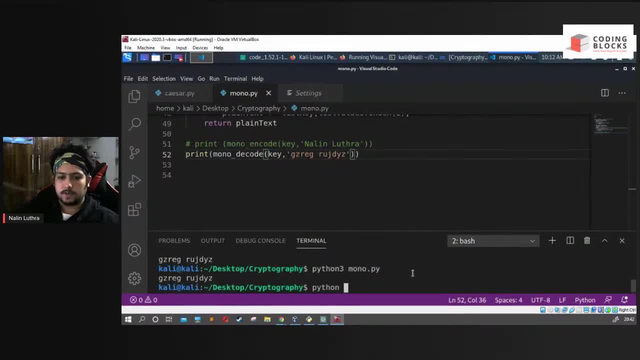 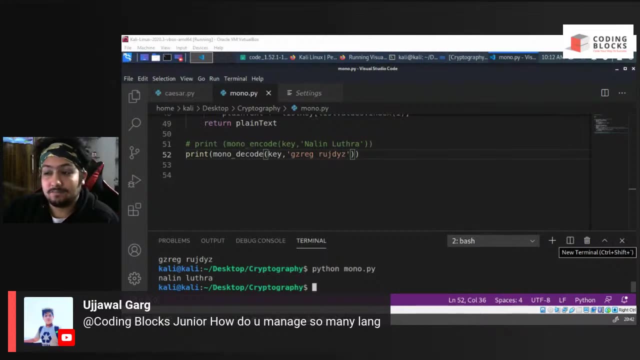 okay, let's save this one. uh, let's run python. py, done it, awesome code word in first time, awesome man. so we did the mono substitution right now. i got some doubts, so maybe i don't know how do you manage so many languages? uh, it's just simply. 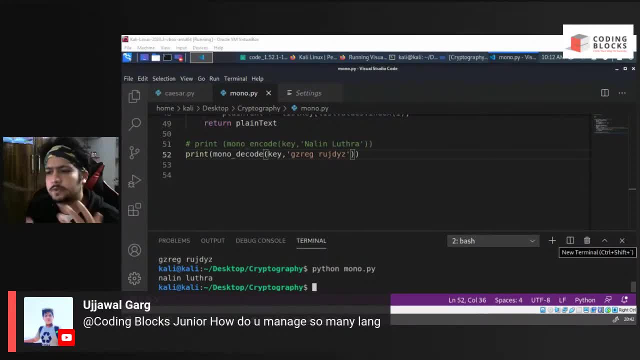 you practice those languages a lot so you get hang habitual with these languages so you're good with it. so i know java, python, c plus, plus- that's same, just a little bit of differences. javascript typescript: that's good. javascript typescript is actually same. uh, when you load many languages, 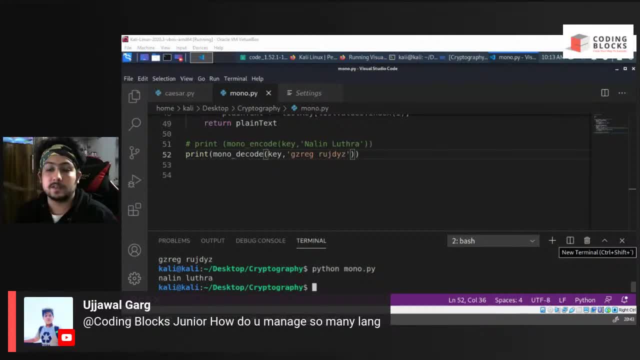 you just get hung of it and you know like everything is kind of the same in many languages, like in case of c and c plus, like in case c plus things are same, because with java and c plus plus things are same again. uh, only like a little bit of differences. uh, just like build out statements. 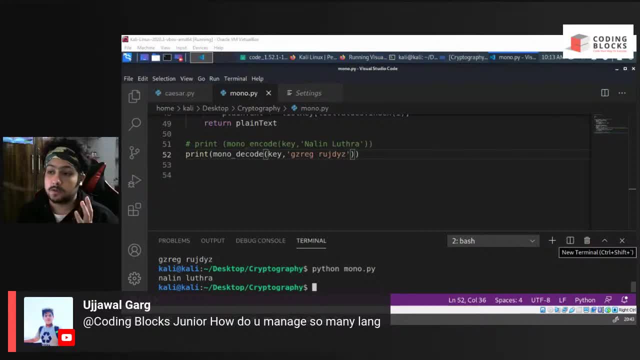 and all stuff like that. then again comes arduino, which is similar to c plus plus and java together, because it's out. uh processing also works in similar ways on java. i don't know what a language is like. go line is cool. so yeah, like you just get hang of the a googling as well in plastic data for. 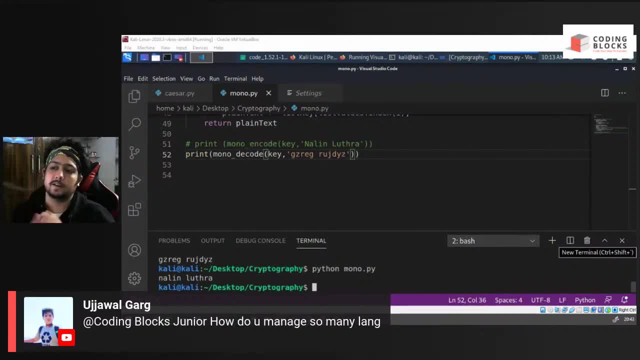 Swift works the same as Python, so that's how you can relate it. What about what are like? so poll, poll is a difficult one. Bash is the same as poll, so we can actually get hung up in time, So let's not go into that. 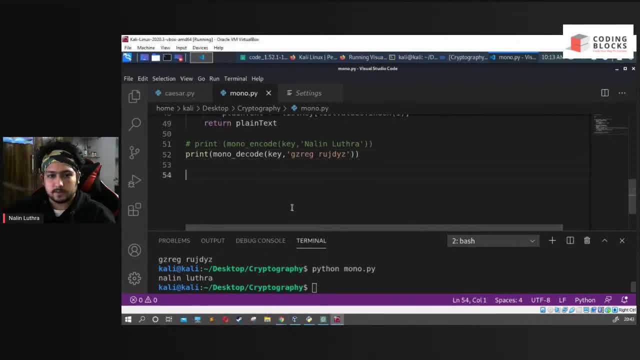 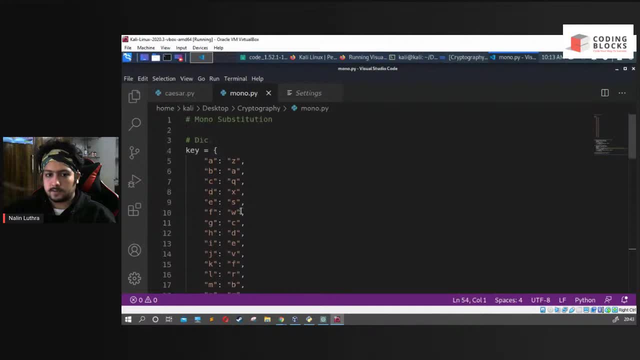 So yeah, you remember the new languages and you've got it done. So please go to explain once again. So yeah, let's explain the code once again. Okay, so this is the dictionary I made. Okay, guys, so how you write a dictionary. 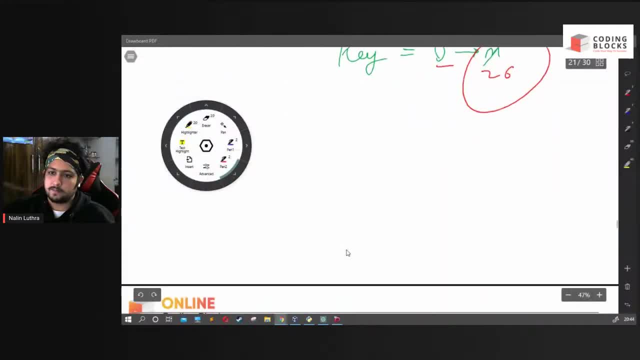 is kind of simple. Let's let me give you, like tell you how I made it. I made dictionary previously for the code itself, So I don't have to waste my time and stuff like that. Okay, so in that case it's simple. 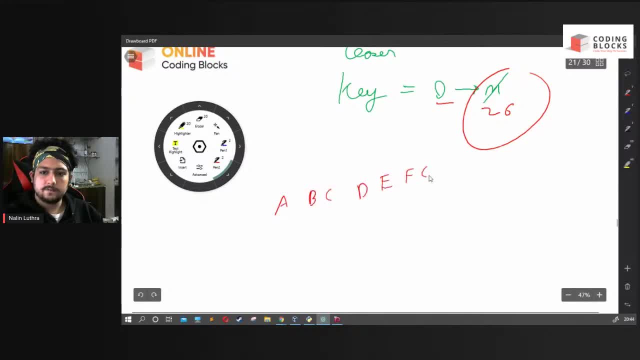 Let's say A, B, C, D, E, F, G, So you write everything you want in paper. After that you just say: A is equal to B, So just cut the B Now. B is equal to C. 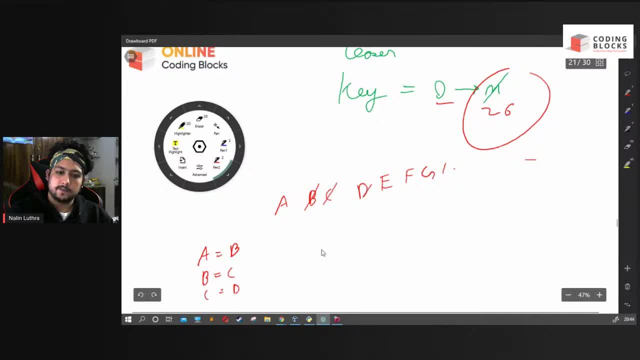 Now cut the C. C is equal to D. Now cut D from here, right? So like maybe let's say C is equal to E. okay, So now you cut the E and so on. So that's how you do it on paper. 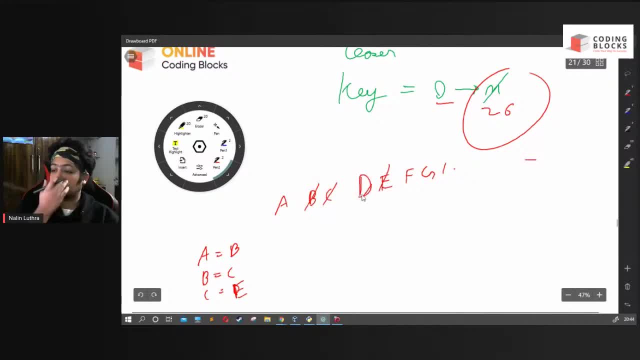 So D, cool. So okay, that's how you do it, And you do this for all the 26 alphabets. These alphabets should go in ABC format and you just cut those from here here here, like this: 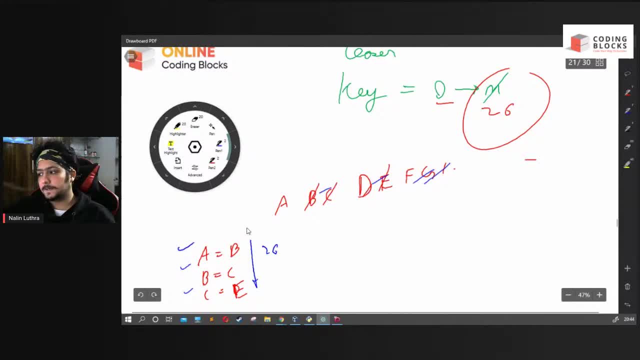 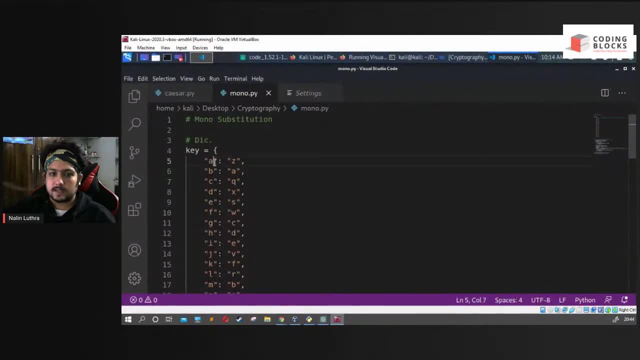 Okay, so that's way, you won't be able to- what do you call it? Miss any letters in throughout the scenario. Okay so, let's get back to it. So that's how I do it. So I take A, I take Z. 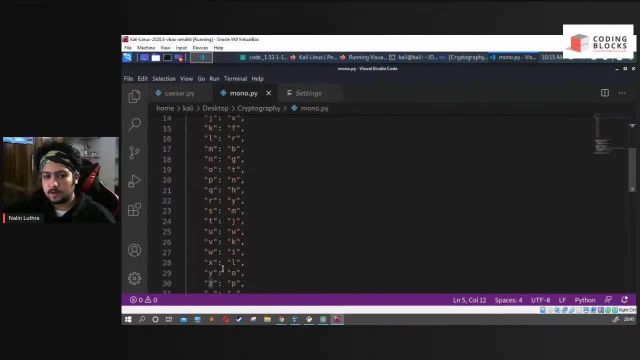 So I cut the Z I take. now I've written ABCD over here like this: okay, After that I wrote those random things which I was left and I just cut this from the paper and that's how you get it done. 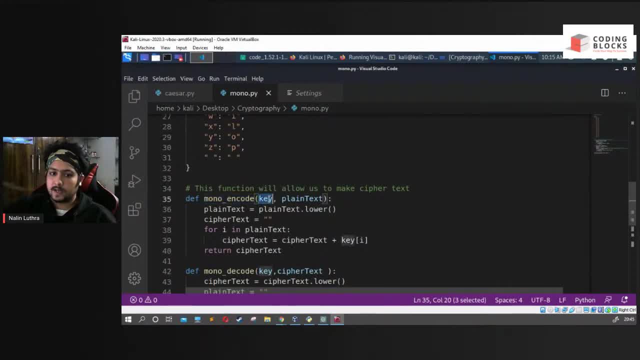 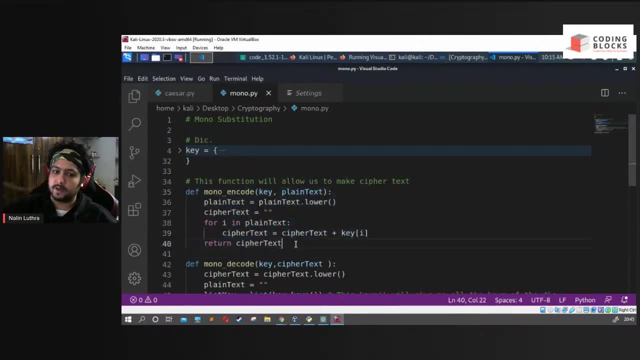 After that, from here, I use mono encode. okay, I pass a key, which is the key. This is the key. okay, This is the key which I made. I will be able to pass this in a function. This is the function I've made. 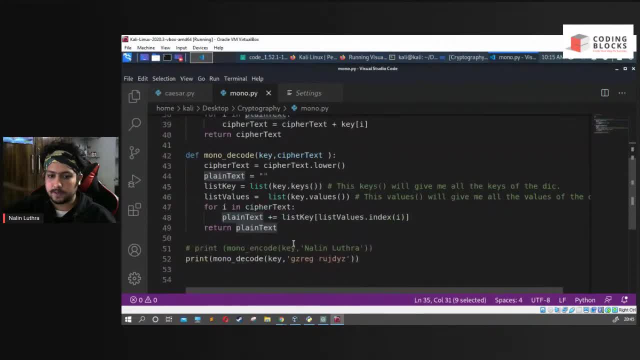 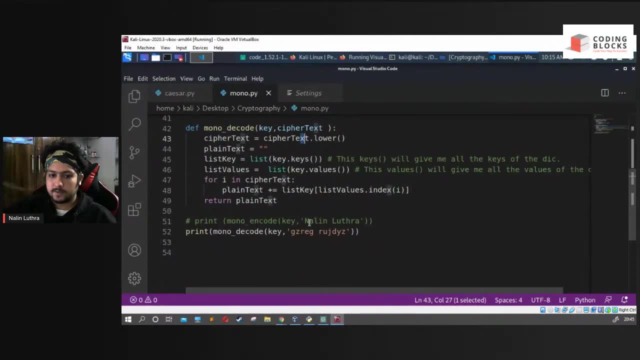 I'm sending a plain text, okay, So let's see what the plain text I've sent. I've sent plain text over here as null and do throw right. So I text a plain text, I make it lower. So when I'm using something as capital N over here. 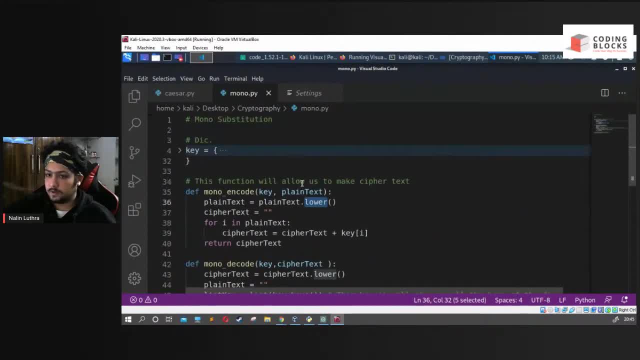 right. so over here it will become lower on its own. Again comes the ciphertext. So I've made a simple plain ciphertext, right. So that's right with Azure, That's right. That's how I'm doing that. Okay, for now I in plain text. 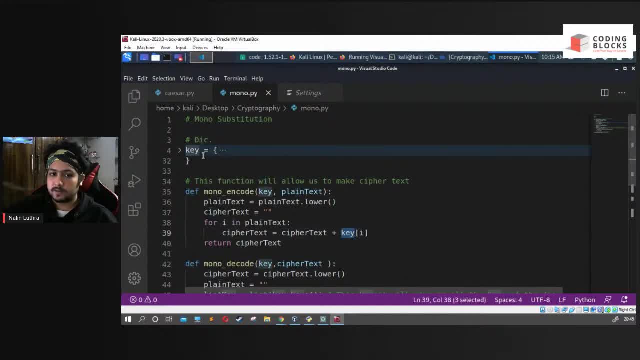 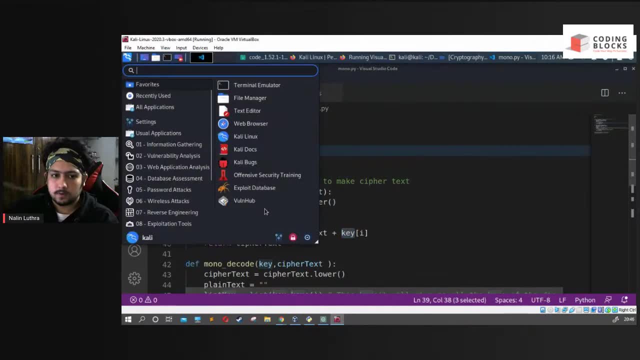 So, like I goes in plain text: We get a key. What is the key over here? This is the key. So whatever I have over here is like this: So do I have an epipen with me? Oh, let me get an epipen. 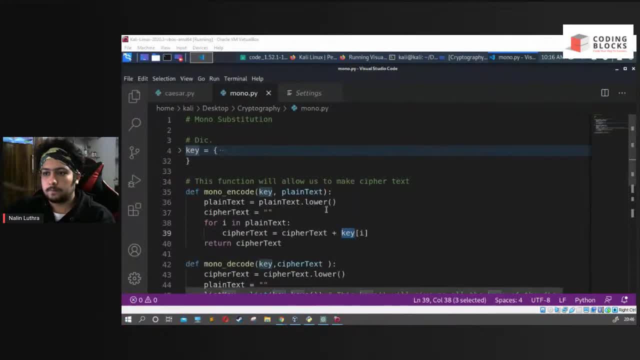 Oh, not this one. Oh, my bad, Cool Going. It's here, My pen is here. No, I don't want to know that. Okay, Let's move forward. Cool, Cool, Yeah. So you see a key over here. 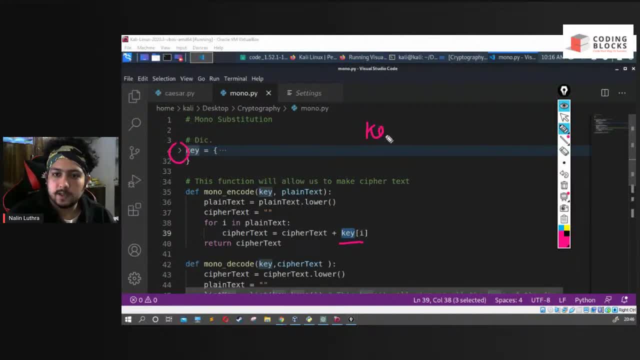 So when I say when I open this one, I will get select key, I give A right, So I instantly get a Z right. that's how it's working over here. this thing, that's how externally works in Python. okay, nice, that's how I'm getting it done. 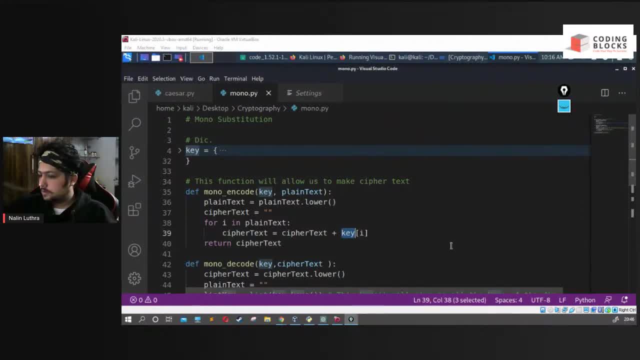 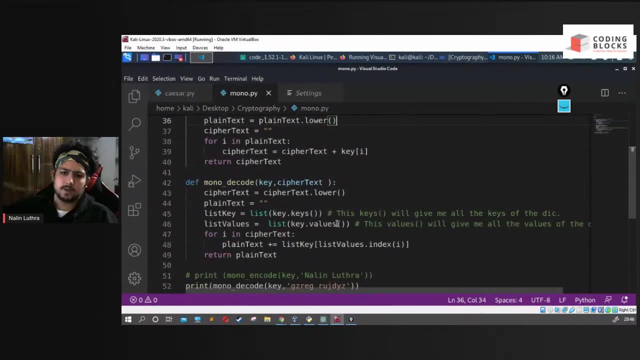 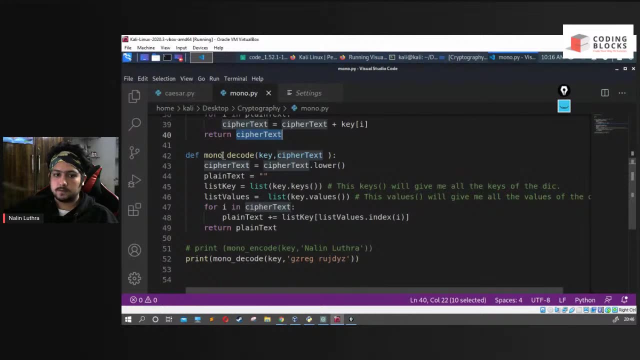 we forward to this one. so that's how I get it done. you know what? I'll tell you something problem I have with college. weird now I just written the ciphertext all together and I use mono decode over here and I use the ciphertext lot, lower list and whatnot. okay, that's all. you get it done. it's done. so up till now we have 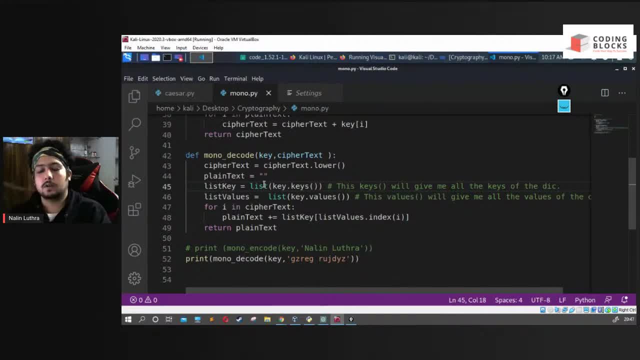 used two different ciphers on Saturdays and Sundays. on Saturday we talked about encryption, everything about Caesar cipher. on Sunday to itself, we talked about with cipher. this is a mono substitution cipher. all these cipher worked by replacing only one alphabet on there together. I can also decode this cipher if I use, like 26 factorial right, so 26. 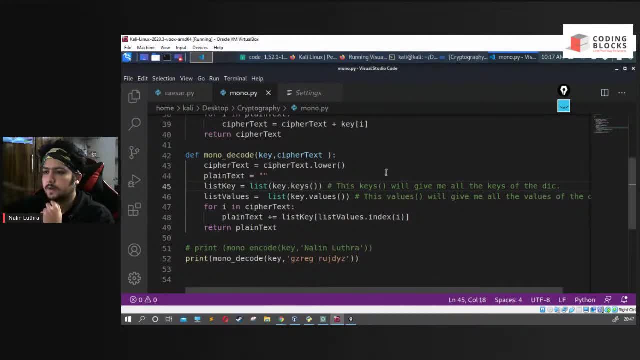 factorial- how big is 26 factorial? let's, let's. uh, if you'd like to code on something or not, I don't know, you just figure it out so we can actually decode even mono substitution as well. it won't be that difficult how you do it, it's. 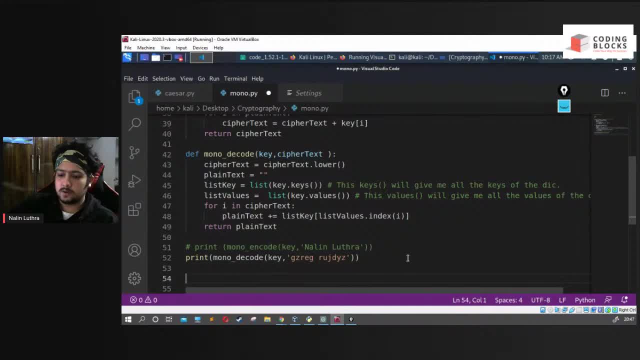 kind of a simple. it's just need how many? like 26 different loops. so I'm just like, let's think about this, okay. so let me give you a sample for it and that's your homework. your homework is to write a code to actually decode mono substitution. 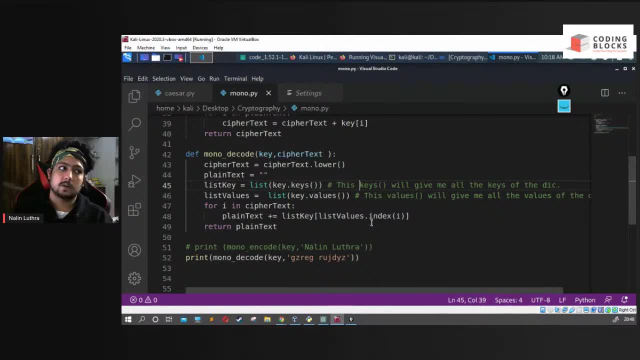 okay, you have to print all that digits which are there, and then you have to find a key out of it and decode it right. I know it could be difficult, but uh, what if, let's say, you have got a paper right on that paper itself? you know that. 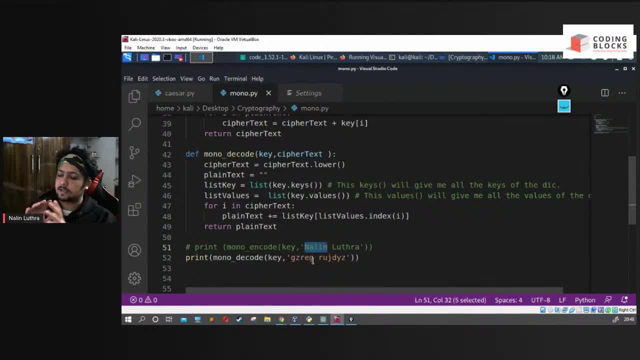 Zekruk means nulling, and that's the only thing you know, and you don't know anything else. you just know Zekruk means nulling. using this, you can actually decode it easily. no, Lakshay, that's not a 2d loop, that would be 26 loop, 26d loop. that's weird. 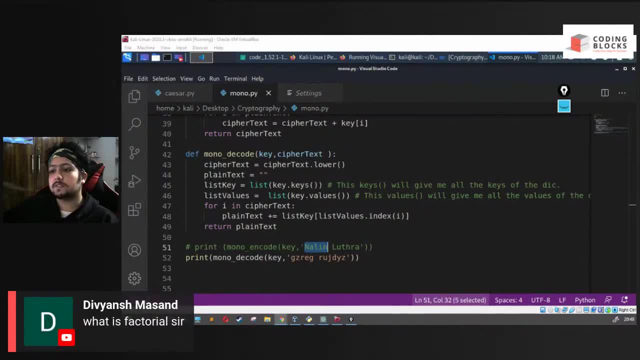 okay, Divanshu, what's factorial? Divanshu, factorial means, if I say 26, factorial, so in 26, then 25, then 23, 23 and select like six. factorial means six into five, into four, into three, into two, into one right five. factorial means five into four, into three, into two, one, so five to four, twenty twenty. 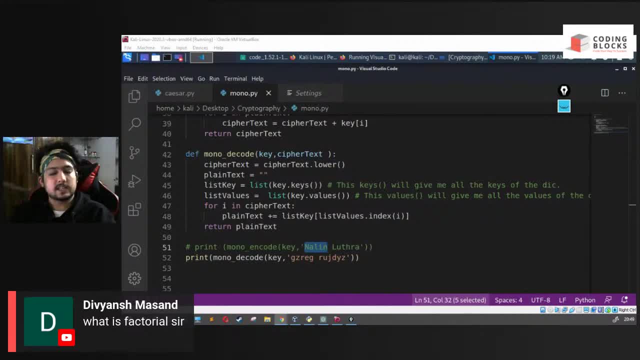 to three. sixty six into two, one twenty, so five. five is 120.. six factorial is 720 central- i don't know, i'm not a genius- and so on. so now you guys have to think how would you decode it when you know kuzruk means nulling and you don't have this key with you. this key with you don't have it. you. 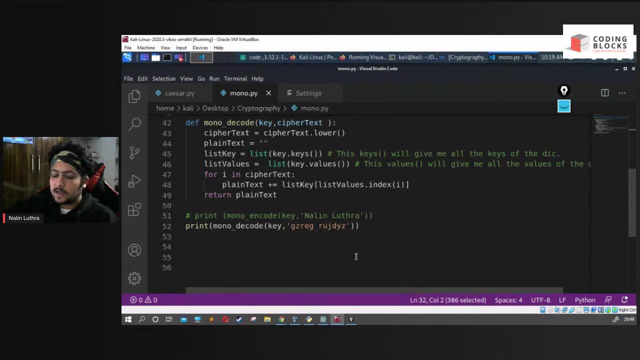 just know: krezik means nulling, and then you have to figure out what does. ruzier means right? you can guess these things, but i don't know. so now you have to do it. you have to figure it out. that's your homework. think harder. i give a good example how to do it. i will just write this one more code: 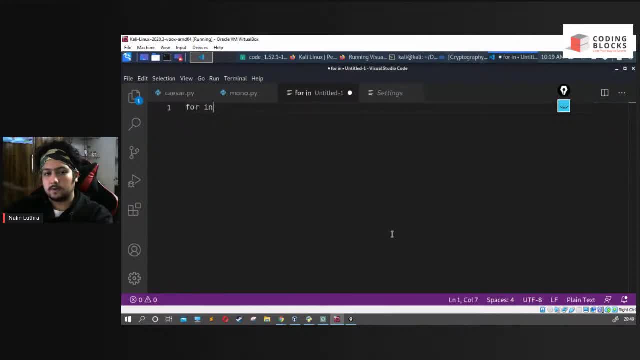 how to do it. i will just say for in, for i, in range 26, that's all, and i will make one loop. let's say a is equal to a, b. okay, like these are letters over here, i'm just giving you a hint. you have to think, guys, okay, this is not the right answer, i'm just giving you a hint. 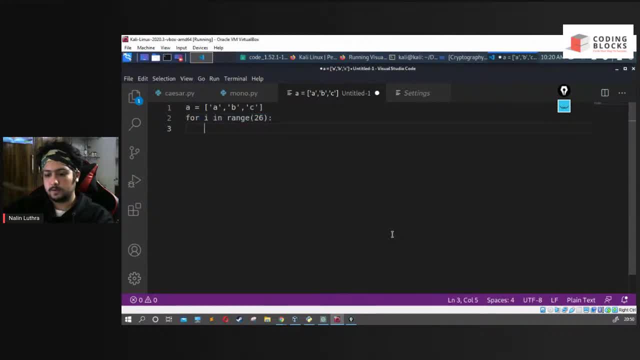 use this for. i now use this for j, k and so on. this list will go up to 26. you can easily check it like if that matches this one or not. that's one way, or maybe you can decrease it a bit. what about taking 25? because no, you when. 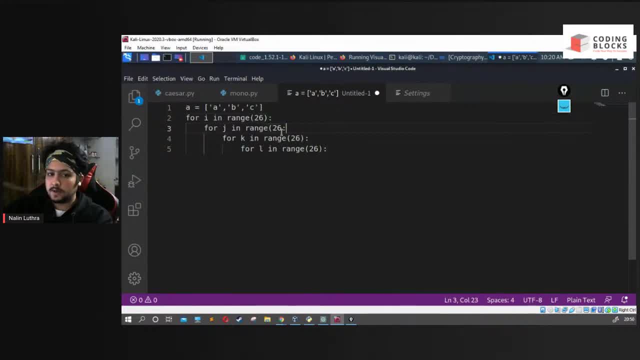 you have a 26. when you don't have 26, you can't Check. it's a capitalpsilon. how about taking 25 one? you don't actually need this one. i don't know, maybe that could be answer for you guys. think about it. how would you actually decipher this? 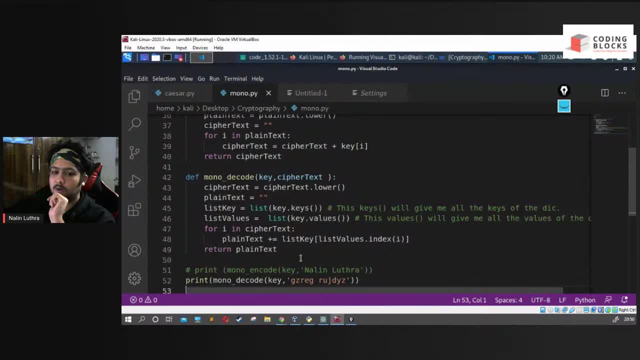 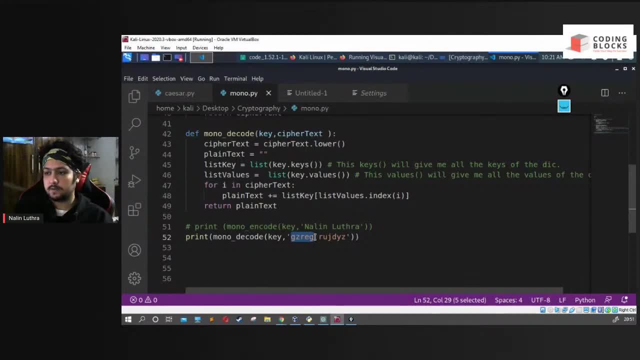 this one without having the key. you only know null in means crescent and that's all. now think hard and decipher, okay, uh, what you guys use. that's completely on you. on the next class, we will go one step higher. instead of going with one substitution, we'll take two letters and do substitution, which is a play, fair cipher. 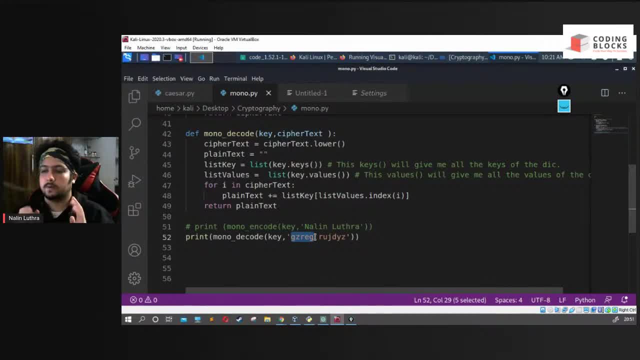 oh, i should not tell you that one because that's a surprise, but whatever, okay, guys, so we will do a different cryptography on the next class itself. so best of luck. uh, and do not forget to decode this, or, if you want, i can send a code. i will upload both the codes in discord itself by today. 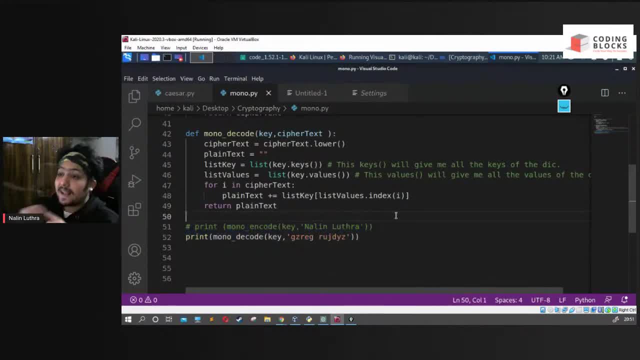 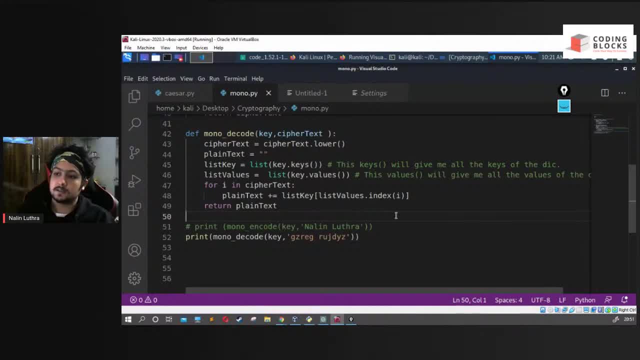 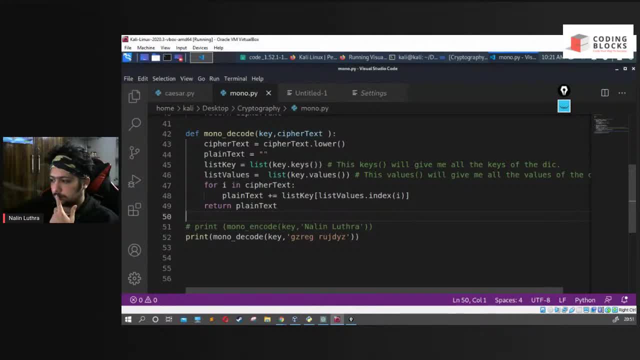 so you, you get ideas about that. yeah, do that. why not go through 26 loops? okay, so that's how you get it done. you get deep, you involve your brain into it and you figure out with something like what. that's the answer, and i want you guys to think about that. 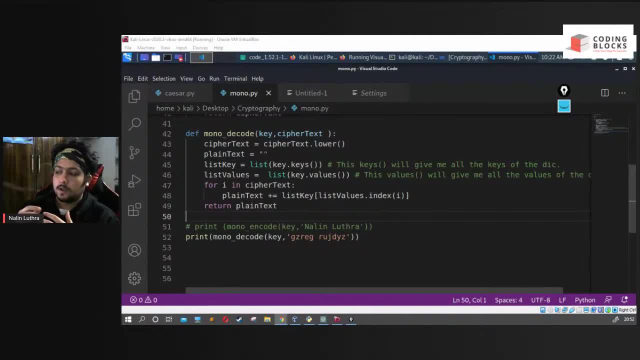 because when we talk about real hacking and real scenarios and stuff, then you should- should be hard enough to actually get to the point where you actually need the answer and solution from. Okay guys, So find a way to not use 26 loops. How you will do that? 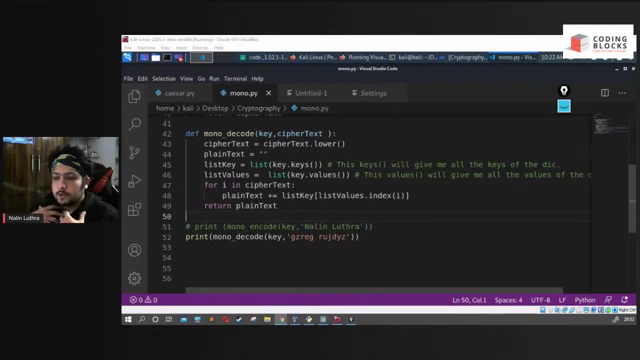 The question can be used: Is it possible or not? Think about it. So you have limitations, you have solutions, you have problems. Now, that's what your brain is used for: to actually think deep inside and come up with an output. 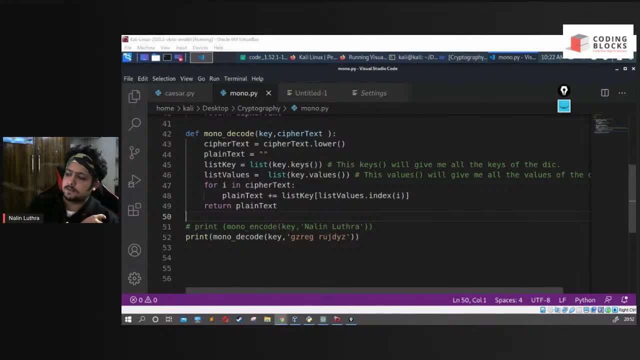 Like you know what This might be the answer, And that's how you build your activities, your thinking capabilities, Right? Those who don't know what is recursion don't have to use recursion. Think from loop, Right, guys. So I think that's all for today. I thought I may. 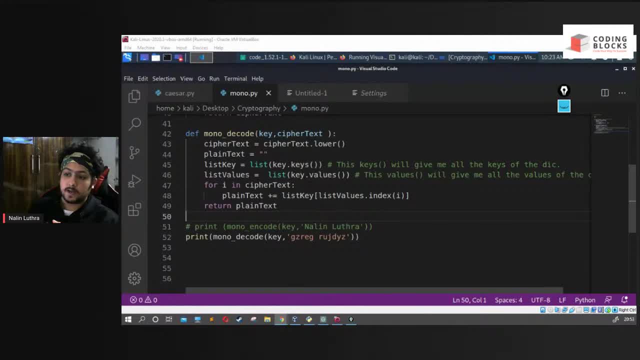 I did thought that I might introduce you a good cipher, a next level cipher, which was actually used in World War II In 19.. I'll tell you where it was used. It was used in World War II in 1854.. 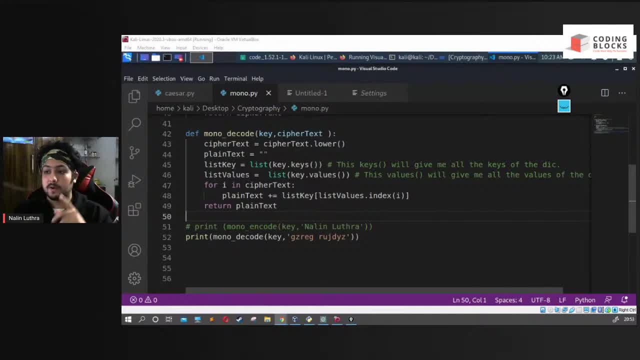 That's right. So there was a cipher which was used in 1854 in World War. Which one was it Like? World War II maybe, Yeah, World War I II, I don't know. It was invented in 1854 and was used. 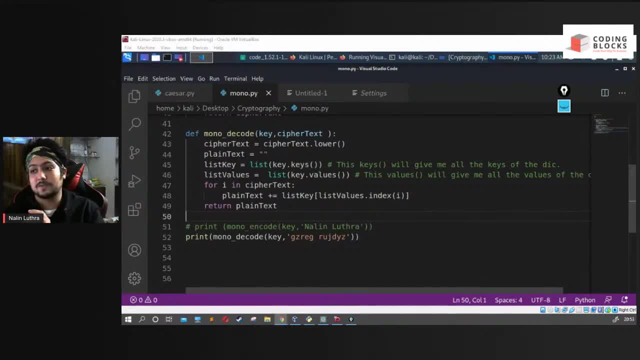 in World War II. So imagine that much hard cipher was because it was not able to be deciphered in World War II. Maybe we will work on that cipher in the next one itself. I won't reveal it. I guess I might have revealed it, But yeah, I won't. 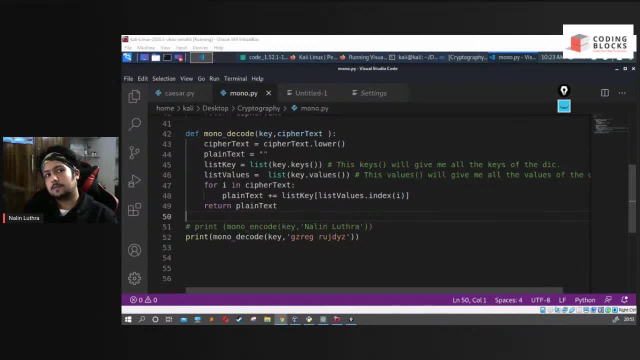 Alright, guys, So best of luck. If you've got any doubt, message me on Discord. I'm not- I'll always be active on Discord, So message me on Discord, I'll give you the answers and everything. Anything you want to come over here. 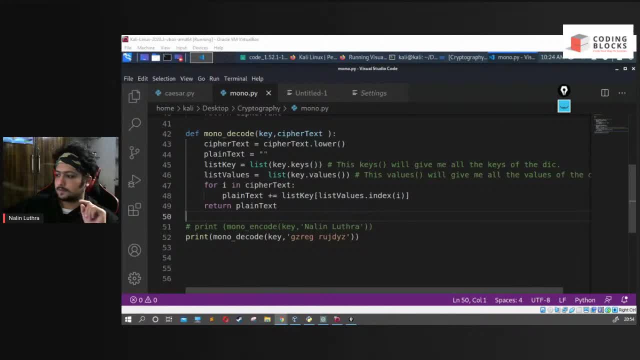 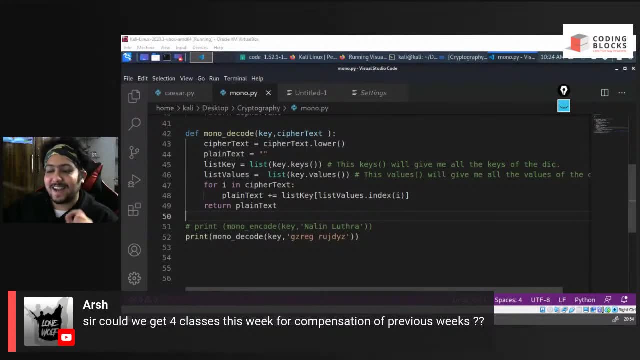 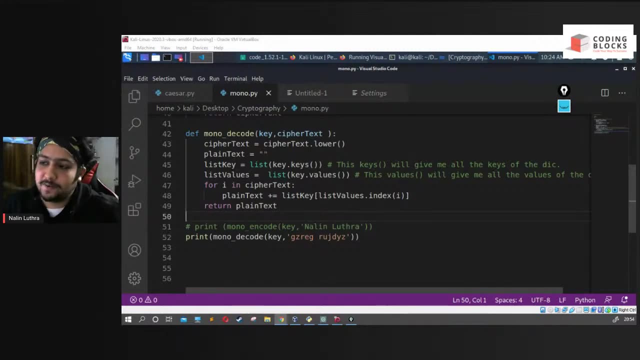 No, no, no, That's not. that's not the one, It's different. No, Ash, We cannot. i don't have so much time, man, so time is the big game over here? no, yeah, we're not actually trying to decoding them over here. okay, now you might be coding. uh, we'll see, we'll see. okay, oh, tani. 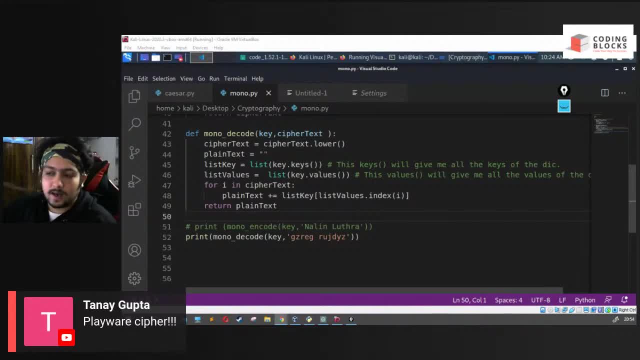 got the answer: it's player cipher and it's not that easy to d. that's fun. that's fun, guys. yeah, then i got the answer: player cipher. that's right. so don't go into that. first of all, first let's decode the mono ciphers and then we'll go ahead. so we will what we have started from back from. 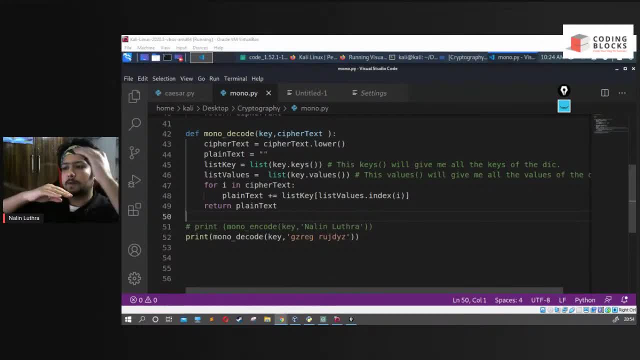 caesar, the basics one, then we got more substitution, then we go to bigger and bigger. and that's how you are to level that these ciphers cannot be decoded. what's way too much decoded like? that's not true. every single cipher can be decoded, but uh, uh. but the point is: 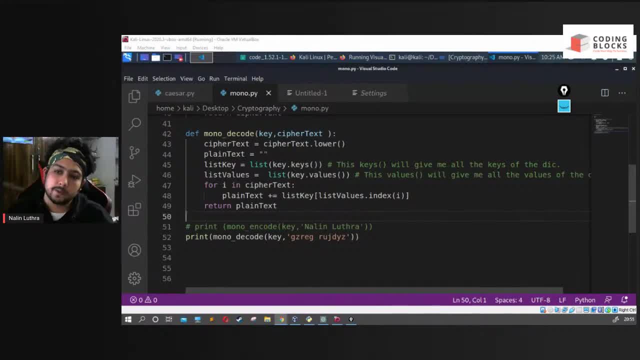 all that ciphers when you decode it. it requires so much computing power that it's not worth decoding it all together. right? so it's not like something is impossible in cyber security and hacking. it's just that it requires so much programming, so much processing power that's not worth getting it done. that's why people change password constantly, so we don't know what. 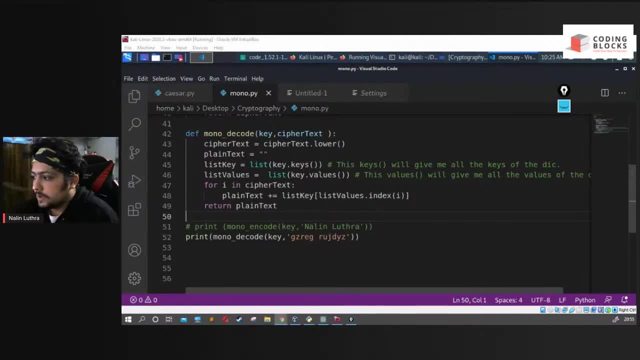 the answer is because, yeah, brute force can be done every time, okay. so okay, let me do a fun fact. you know what you can actually decode or you can actually find answers from brute force using anything on the world. that's why, on big computers and backing systems, the people those actually know 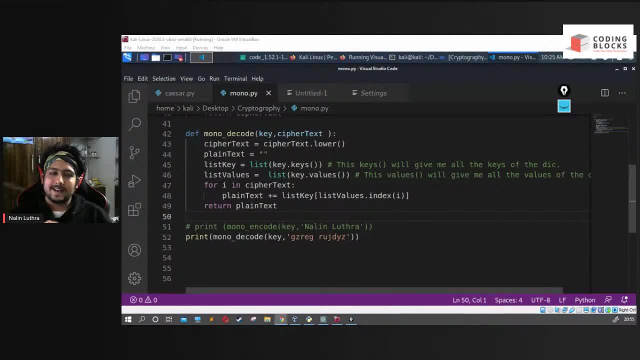 the output and solutions, 20 in within the span of 14 to 15 days. they change the password and the password is usually about like 25 to 30 digits long. that is long. so 30 characters long password gets changed every no, no, no, they did not use it in 1945. no, no, no. what i said was: uh, wait, let me.